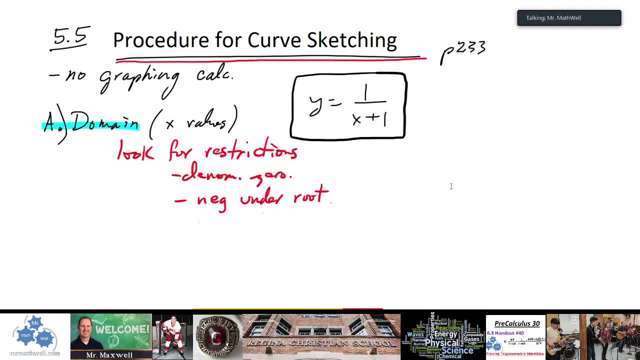 chapter and we're going to put it all together so that we can take a look at an equation like this And, without any graphing technology, we're going to be able to draw a very accurate, very precise graph with all the intercepts and all the asymptotes and all of the maxes. 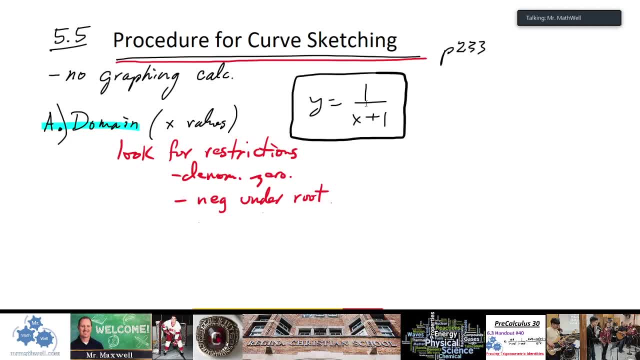 and mins and with all the intervals, concavity and everything, we're going to be able to draw a pretty accurate picture for any function. So there is a list. There's a list of headings or points and in your textbook they refer. 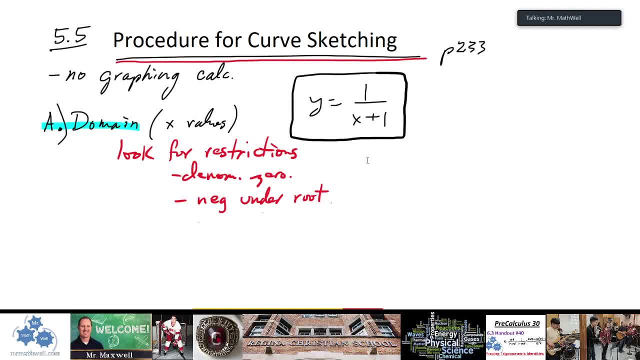 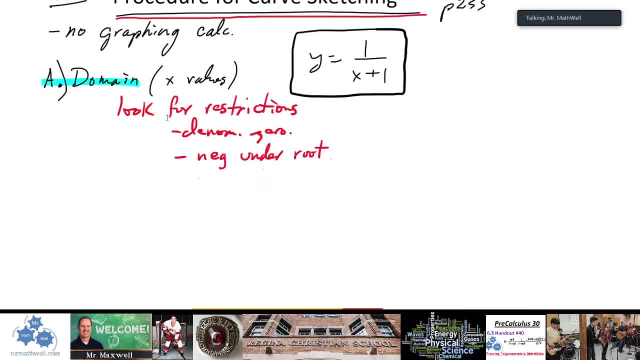 to certifications. So we're going to start with A to H, I guess A to H, And I'm going to go over each one, starting with A. I have a little setup here. So A is domain, B is intercepts, You don't. 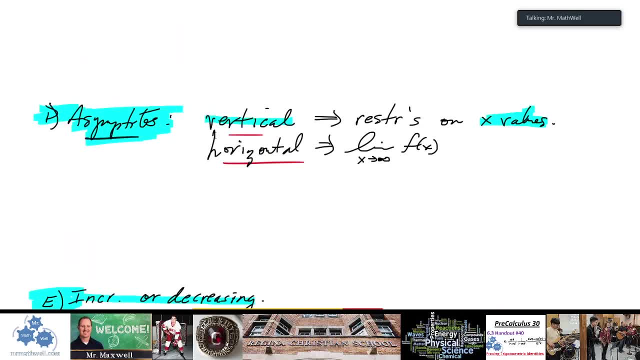 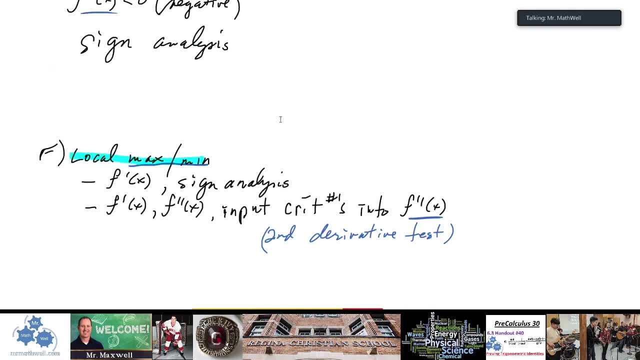 have to write this down now. Just this is what's coming: C is symmetry, D is asymptotes, E is increasing and decreasing sections of the graph, F, local maxes and mins, G, concavity and points of inflection. And then H is sketch the graph. 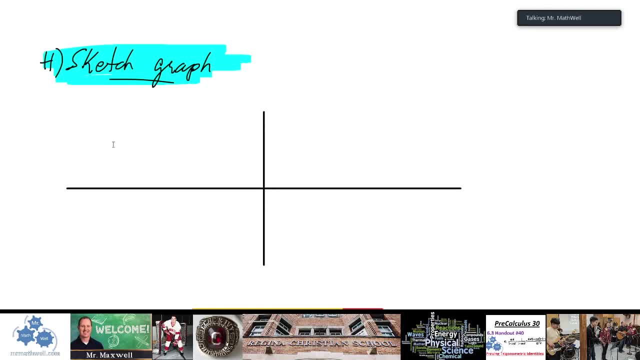 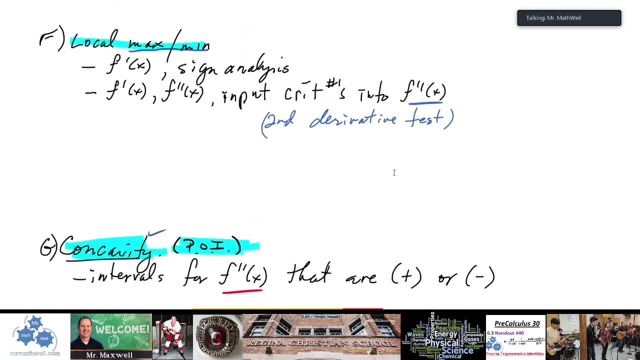 So those are the points, And if we kind of follow, take a look at each point, we're going to be able to accurately sketch our graph. Now in the textbook they get you to sketch the graph once you've determined everything, But I like to sort of keep a running sort. 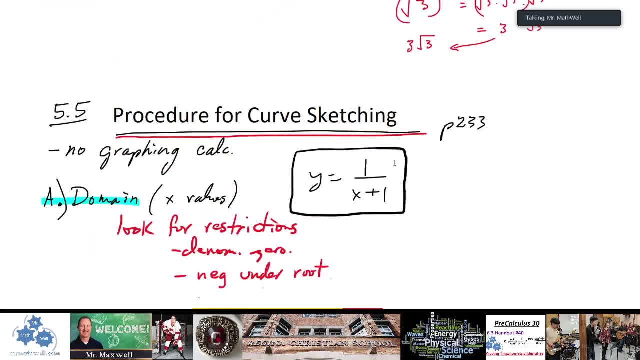 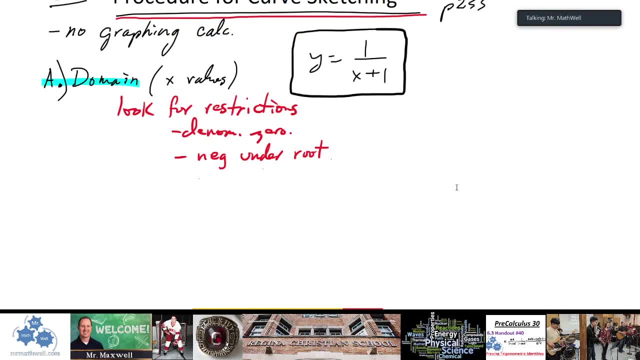 of I like to sketch while I do these points, So I might just try and do that as we go. So I might refer down to that graph And, if you have like a, at the bottom of the page or on the next page, if you just have a. 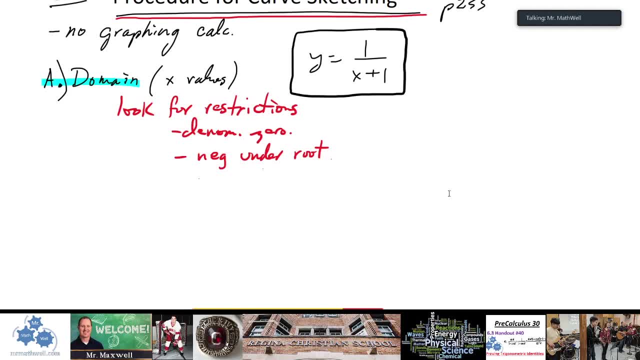 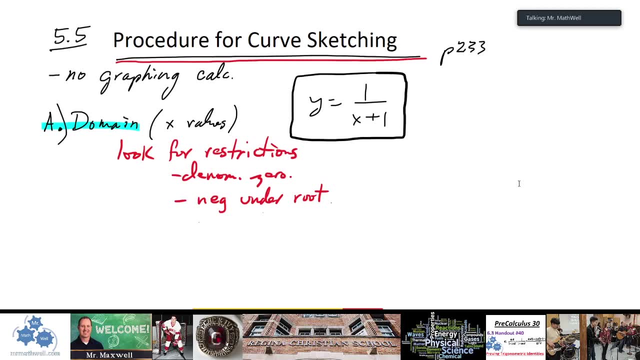 coordinate plane and you want to graph this as we go along. that might be a good idea too. You might like that better, Okay, So, first of all, domain. Okay, So A is domain And I will give you a list of these points. You don't have to memorize these. but so A is domain, So we want. 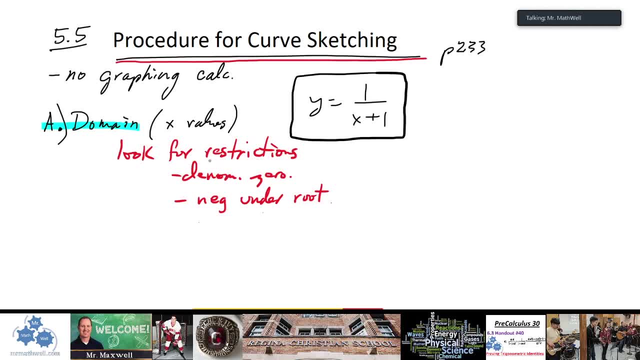 to find out what X values are restricted for our function. Or, if it's a polynomial, maybe we can say that the domain is all values of X. Well, in this case, we know that there is an X value. that's going to be a problem And that's going. 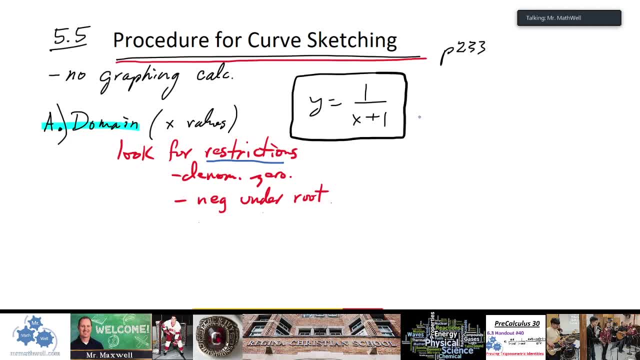 to be X equals what? Well, if X equals zero, we have one over one, and that's okay. but the denominator can't be zero, So X can't equal negative one, Right? So we have a problem where X, X cannot equal negative 1.. Now for the domain. I'm okay, actually, if you state: 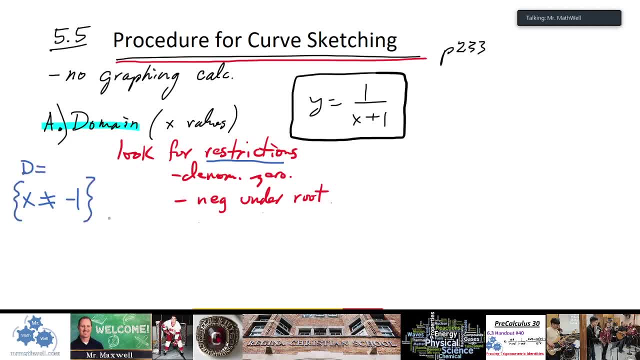 this in the negative like this: what the domain can't equal- I'm okay with that Domain- is: x cannot equal negative 1. We're not really stating the domain right, But that's going to be okay for now. How you might want to do it is you to be, I think. 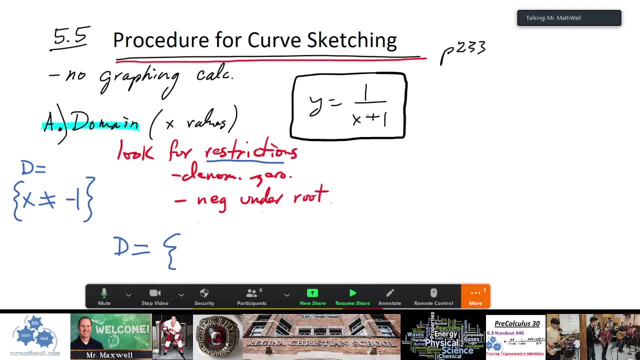 to be totally accurate would be: you would say that the domain is everything from negative infinity to negative 1, in union with negative 1, and not inclusive, of course, to positive infinity. That would be stating the domain in the positive. Okay. 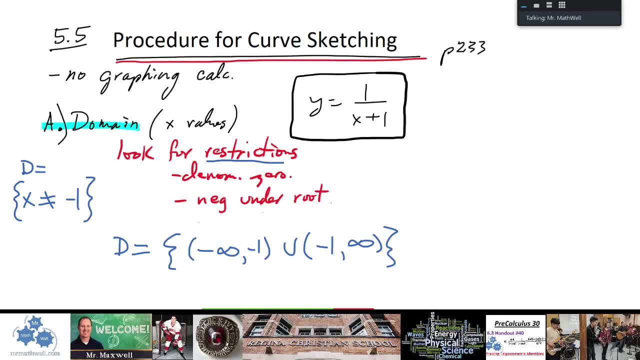 So you're stating everything except negative 1.. So either way is totally fine, with me, I'm fine. So the restrictions: again, the denominator cannot be 0. You cannot have any negatives under the root. That's what you're looking for for domain. 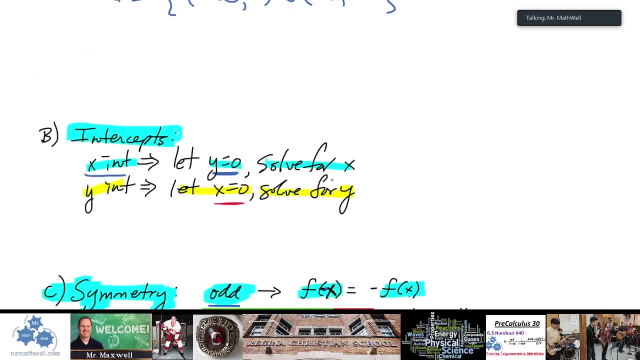 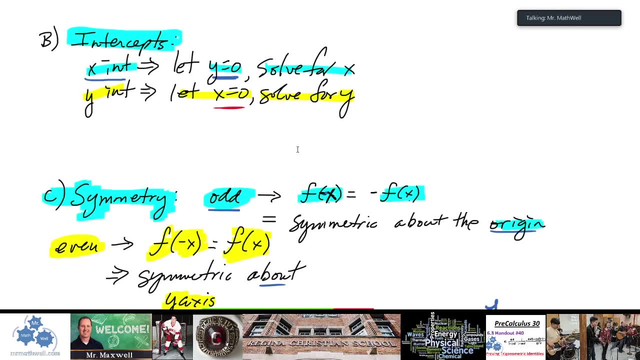 All right. So A for most, pretty quick. A is pretty quick for most functions. Okay, B intercepts. Now to find the intercepts. we know this. We looked at this at the beginning of the chapter. For the x-intercept, let y equal 0 and solve for x. 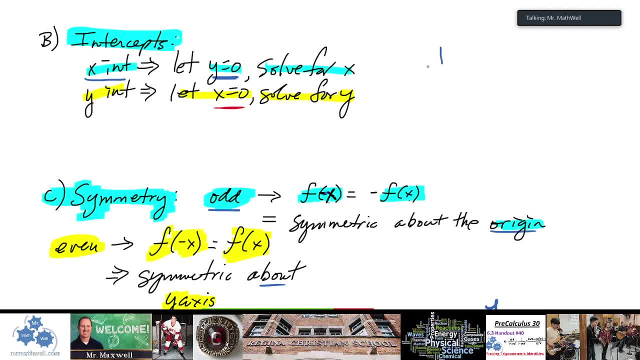 And for the y-intercept vice versa. Let x equal 0, solve for y. So 1 over x plus 1 is our function right, And so if I let x equal 0,, I have y equals 1.. 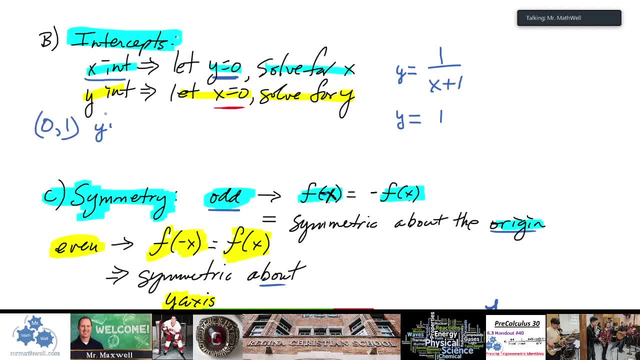 So 0, 1 is the y-intercept. Okay, And if I let now, if I let y equal 0 and solve for x, what do I have? Oh, I have a bit of a problem actually. How do I know that? 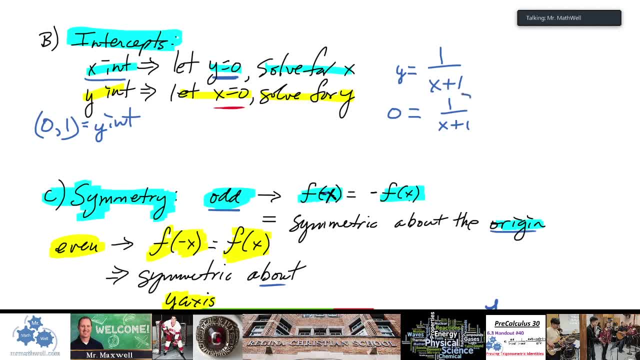 How do I know I have a bit of a problem? Well, because this will never equal 0. Because there's no variable in the numerator. Okay, So 1 can never equal 0. So I know I have a problem. Now, if we, let's say, we multiplied both sides by x plus 1, if you want to do that, 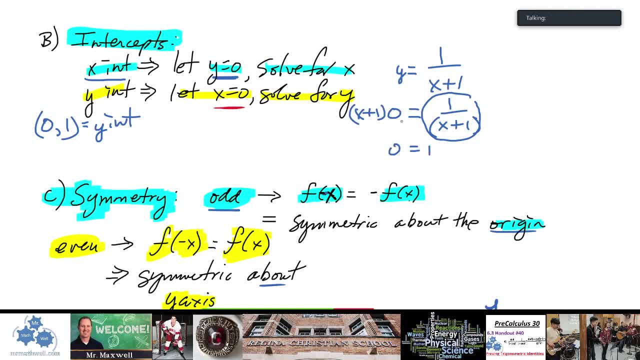 Well then I get 0 equals 1.. That's no good. So there are. there's no x-intercept, Okay, x-intercept none, And that's okay, because we might have some kind of horizontal asymptote there, right? 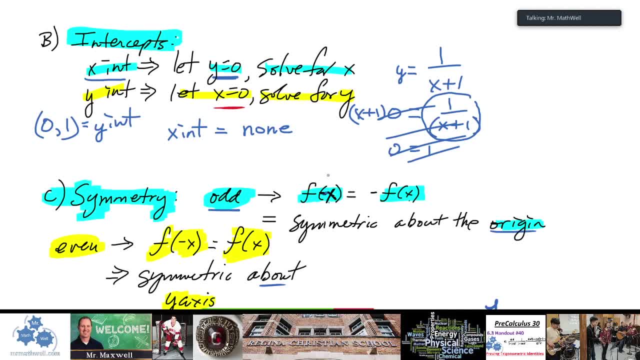 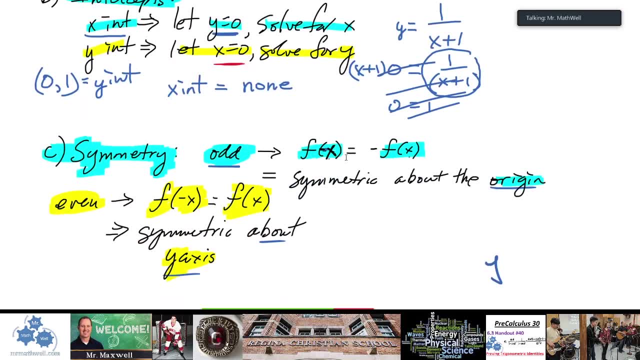 Which would mean the graph would never touch the x-axis. So you kind of have an idea that that might be the case. All right, so that's A and B now, And you know what, If you want to go down to your graph, because what we know so far, 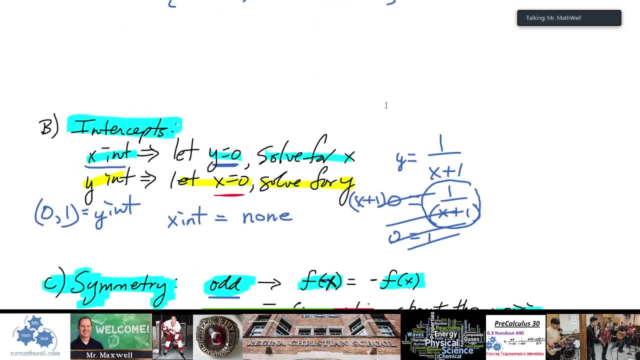 we know that x equals negative 1 is an issue We have, do you know? well, we're going to find out exactly what happens at x equals negative 1 soon, But I know that I have a y-intercept of 0, 1.. 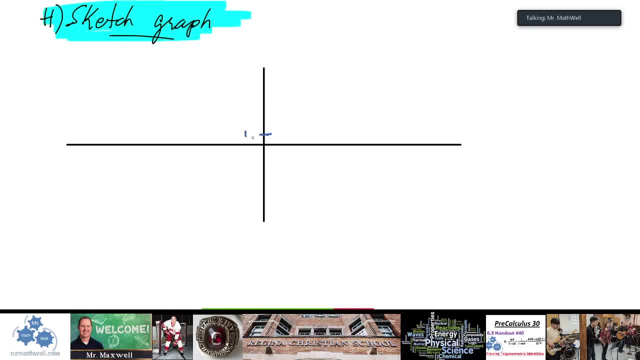 So guess what I'm going to do this right away. I'm going to put this is: 1. I have a y-intercept. I'll do it in red here. Here we go. That's a point I have in the graph. 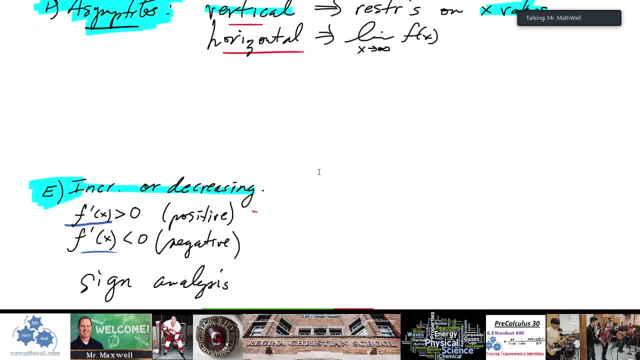 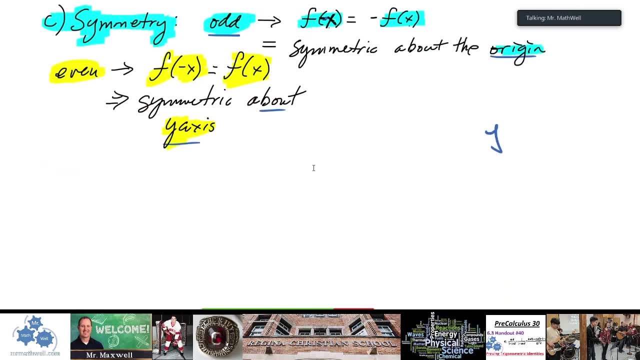 If you want to keep a running total of the things that you're identifying about this graph sketch, then feel free. Okay, symmetry. Well, we learned about symmetry way back when, And do you remember even odds? So odd is when we substitute a negative value in for x. 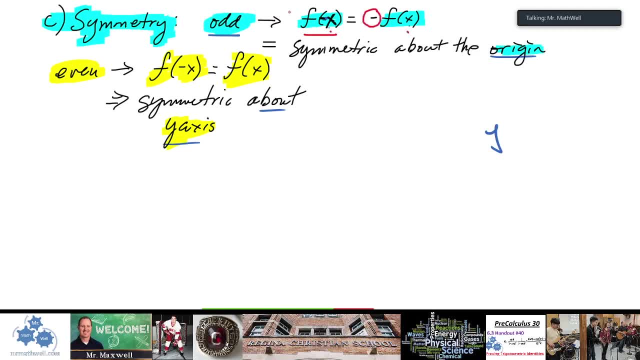 and we get sort of the opposite. So answer: one's positive and one's negative. If we substitute a negative value and it's positive value, we should get the exact same. if it's even And anything else, then it's. there's no symmetry. 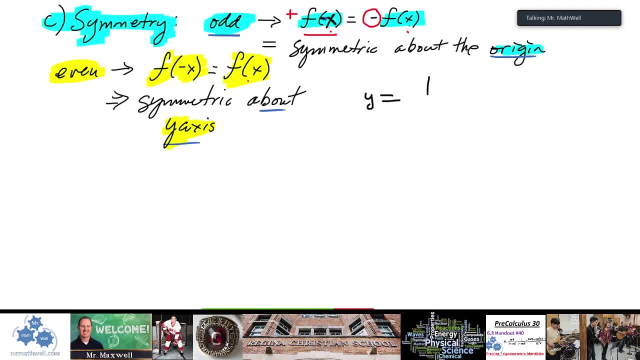 So let's do that real quick. So if we did y equals 1 over and let's pick, well, we can't pick negative 1.. That's an issue, Let's pick 2.. So let's say x equals 2 and x equals negative 2.. 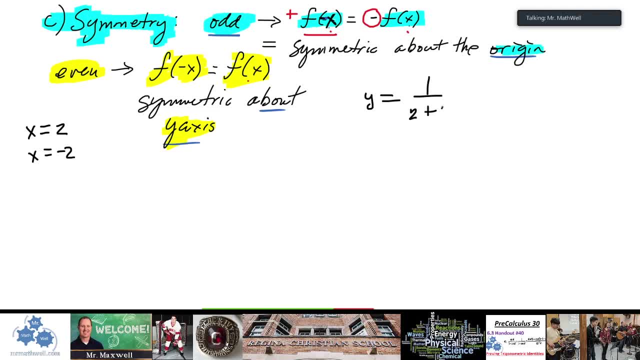 Let's try that. So if I have 2, 2 plus 1. That's y equals 2., That's y equals 1 over 3.. And if I do negative 2, 1 over negative 2 plus 1,. 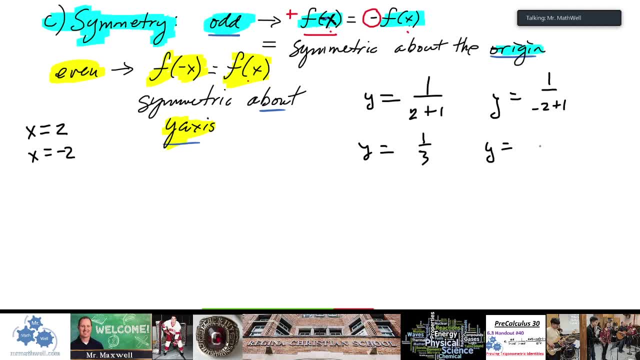 and flag me down if I'm writing anything incorrectly. Sometimes I jot something wrong down, but let me know. But 1 over that's going to be negative. 1, right, So it's going to be negative 1.. Okay, Does that look okay? 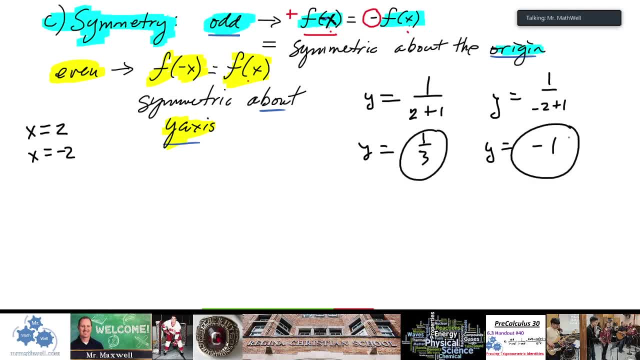 What I notice is that these numbers are not the same and they're not the same value, but opposite sign. So I have no symmetry. So there's no symmetry here, Which is okay. There's no symmetry- at least there's no symmetry about the origin. 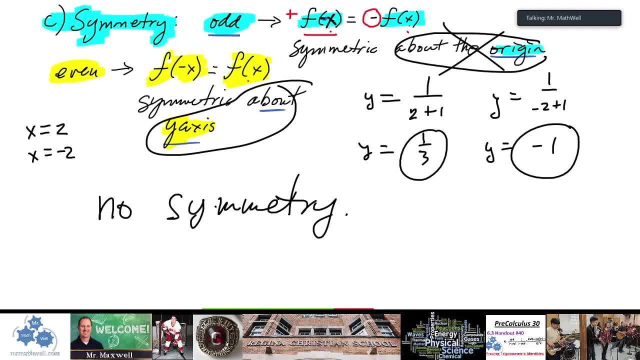 Not about the origin, And there's no symmetry about the y-axis. That's the symmetry that we don't have. Okay, So we may have some kind of generally symmetrical looking graph that's shifted over to the left or right, or up or down. 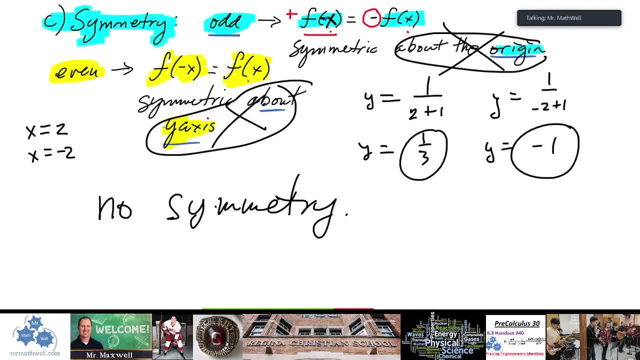 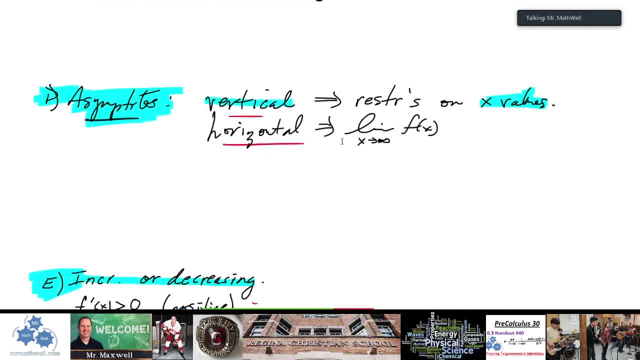 We could, But there's no symmetry about the y-axis or about the origin. You good with that? Okay, Nothing really to draw. there We're on the graph, So let's keep moving on. Asymptotes, Okay, Asymptotes. 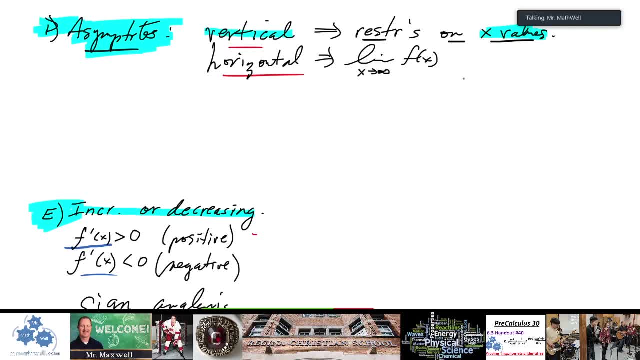 Vertical asymptotes. Okay, Look at the restrictions on the x values. And we said that x. there was a problem when x was negative 1.. And of course, we understand that this is a factor that cannot be simplified out. Therefore, we're going to have some kind of asymptote at x equals negative 1.. 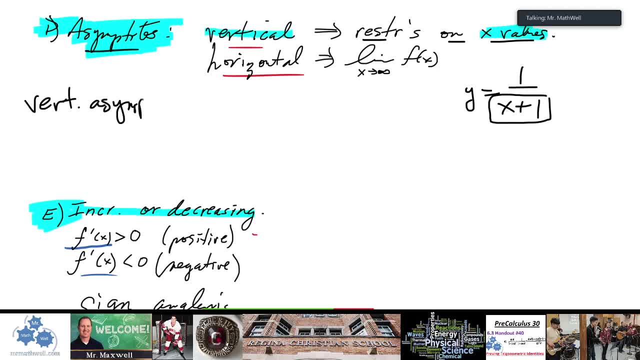 So vertical asymptote right At x. At x equals negative 1, right, That means there's an asymptote. Now if you wanted to check to see what the behavior around that asymptote is, then you could do that. 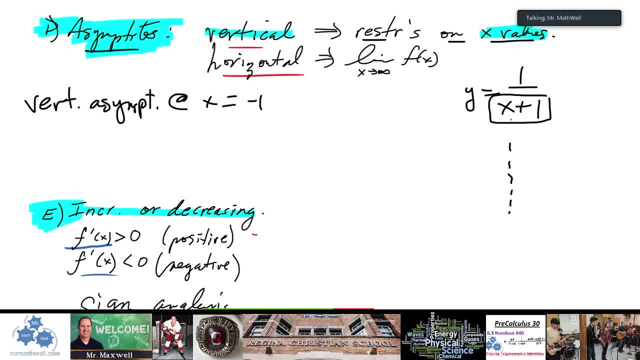 And that's what we did in I don't know 5.3 or something You know as the limit as x approaches negative 1,. what happens here? So if x was just before negative 1, like negative 1.001 or something, then we would have. 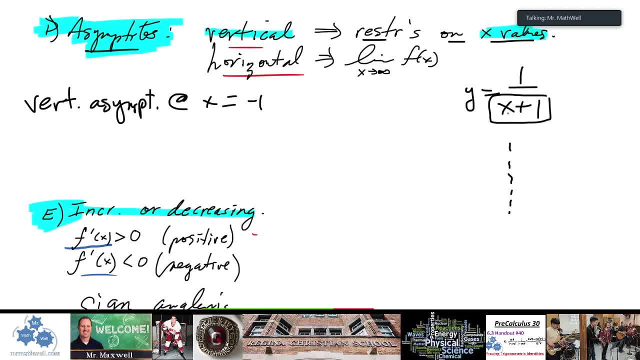 a small negative number, right, And so it would be approaching negative infinity the graph. And if we were approaching negative 1 from the other side and we had a very small positive number, then that would 1 over a small positive number would be a large number. 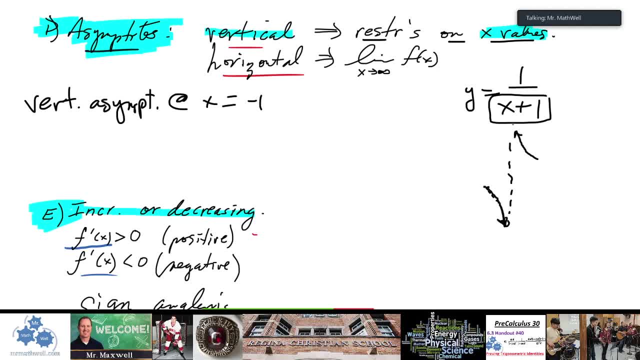 So this is the activity of the graph on either side of x equals negative 1.. Okay, And again, I just substituted values for x and did an estimation. Okay, But you don't have to put that on there right now, but probably at: x equals negative 1,. 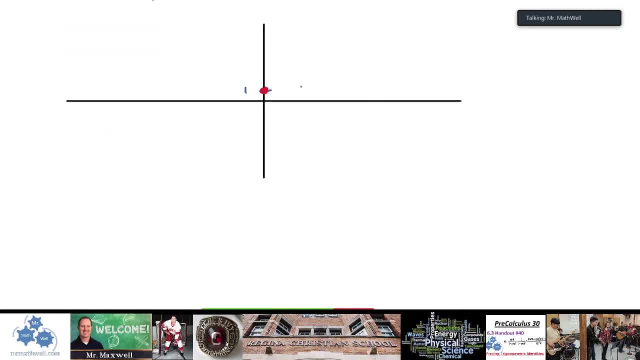 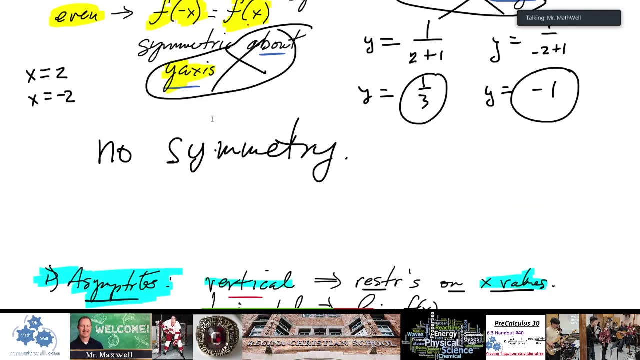 let's put the asymptote anyways and we'll have an idea of what this might be. So x equals negative 1, I'm going to draw a just to express a vertical asymptote there. Okay, Shout out any questions, those of you in my class here. if you have any questions right now, anybody. 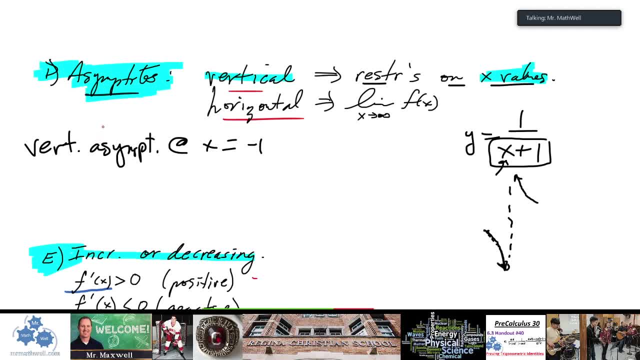 Okay, I guess horizontal asymptotes. This is where we're at next. So horizontal asymptotes, let's take a look at that And remember. that's the limits, Remember the limits. So what is the limit? as x approaches, let's say positive infinity. 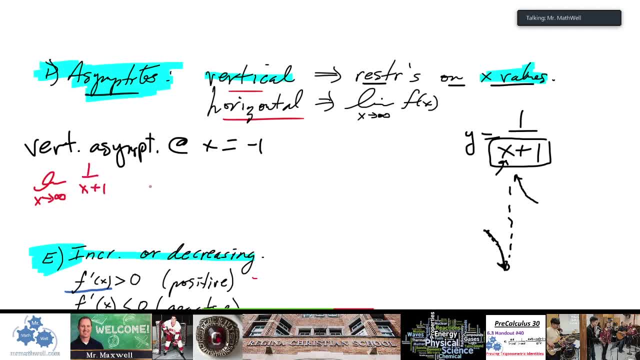 See what happens of 1 over x plus 1.. Well, how we did that was we divided every term by, in this case, x, And so it looks like this: I have 1 over x on top, I have 1 on the bottom plus 1 over x. 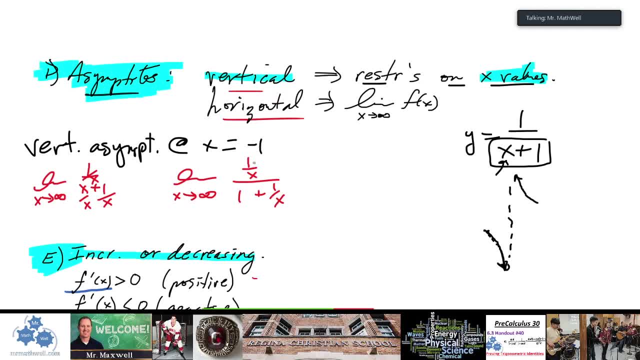 And so if I apply the limit to each term now, as x approaches infinity, that becomes 0, right, 1 over a very, very large number approaches 0. And this becomes 0 as well. So I have 0 over 1.. 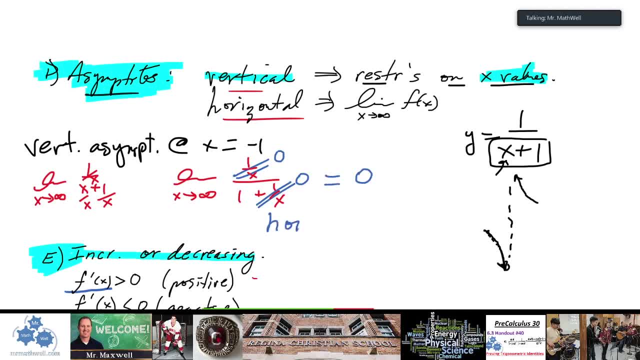 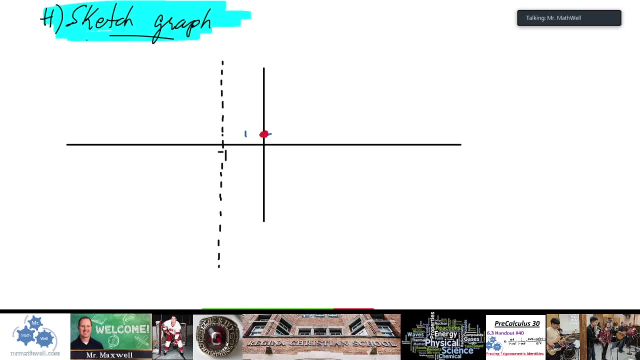 So my limit here is 0.. Therefore, my horizontal asymptote is: y equals 0.. Okay, So if that's the case, then probably what we're going to do is we're going to go down to the graph here And we're going to draw, you know, a horizontal asymptote along the x-axis as well. 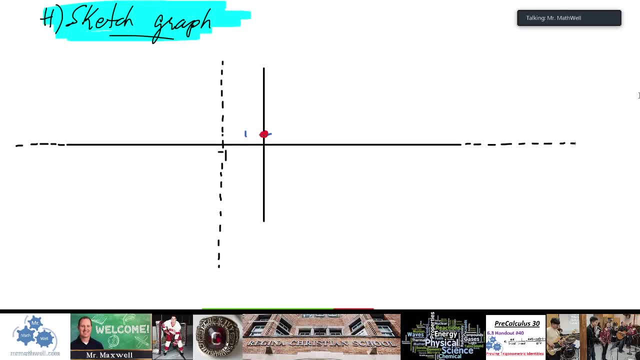 Okay, So this is what we've got so far- Awesome, Okay. Now notice- Notice this- that I've got a y-intercept up here at 1.. Now, if this graph probably is not going to cross the y-axis, 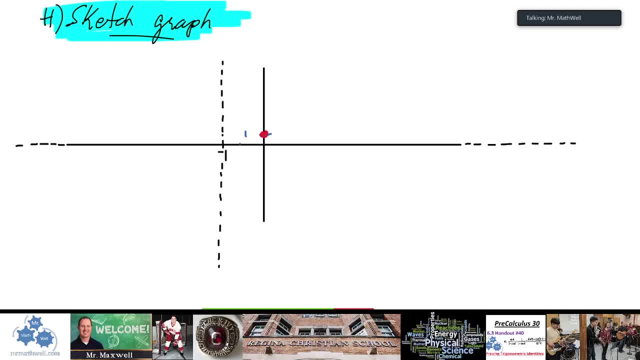 It could cross the y-axis in the you know around here. maybe It could. It could maybe go like this, But remember we did some test runs there about what happens when x approaches negative 1. It looks like the graph is up here. 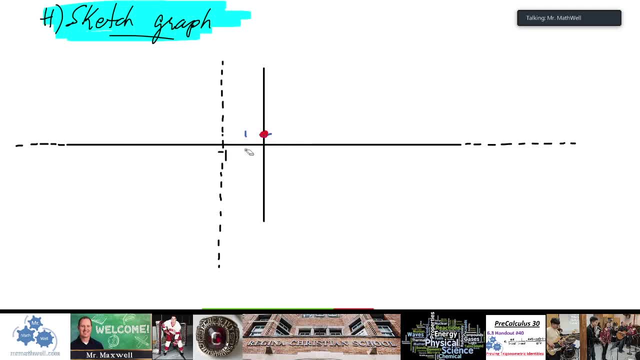 So it looks like it's going to connect through here. What would be nice to know is if we have any x-intercepts at all, Because as x approaches positive infinity, we know that there's a limit of 0. But we don't know what happens in the middle here. 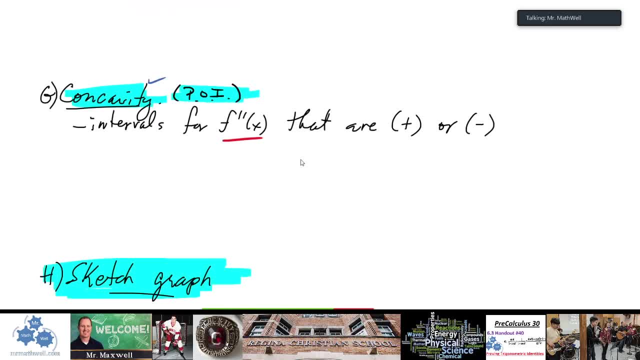 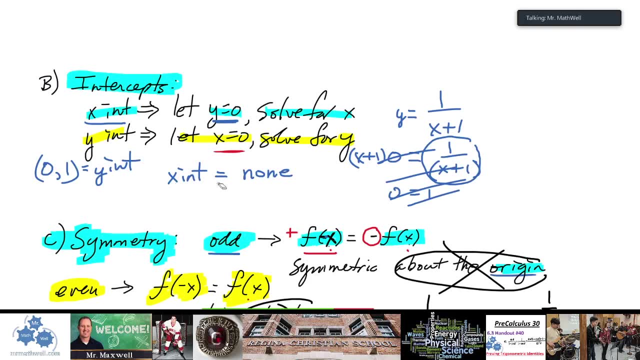 So that's where the x-intercepts come in. Let's just see if there are any. I think that's. Or did we do that already? Sure, we did already. There's no x-intercepts. Look at that None. So here's what I'm saying. 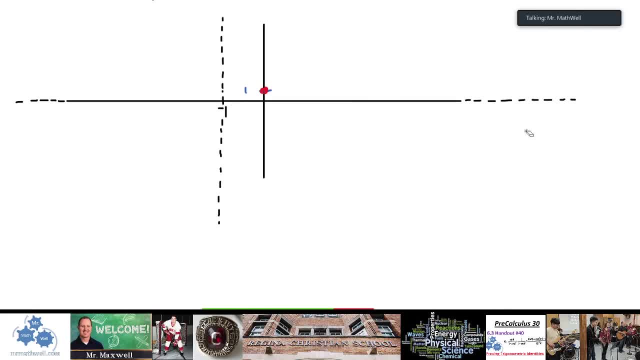 The graph is not going to cross the x-axis out here because as x approaches infinity there's a limit, And it's not going to cross anywhere around here Because we didn't identify any intercepts. So I've got my graph so far looking like this: 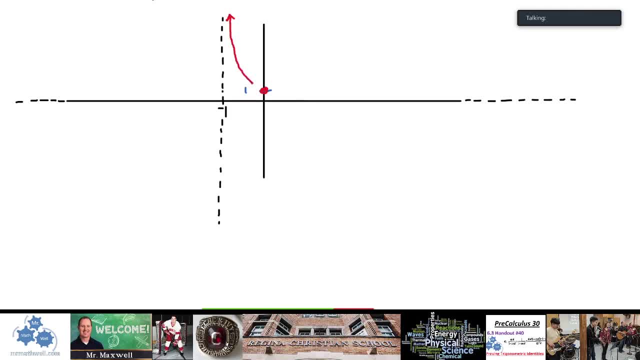 It's got to look something like this. I think Now could there be. Could it go like this? Oh, I guess it could. So that's going to come later when we talk about maybe local max and mins, But it kind of looks like I've got this so far. 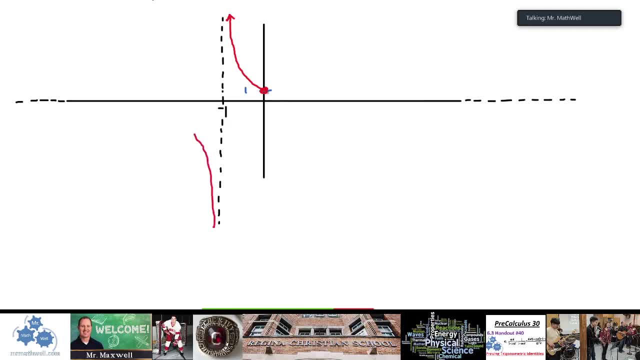 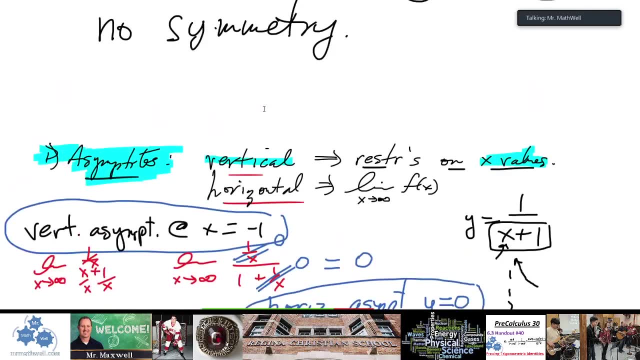 And again you can keep kind of a running total here, A running sketch. So no intercepts on the x-axis. We've got some asymptotes, Let's keep going, Okay, Increasing or decreasing. Well, now we have to take the first derivative. 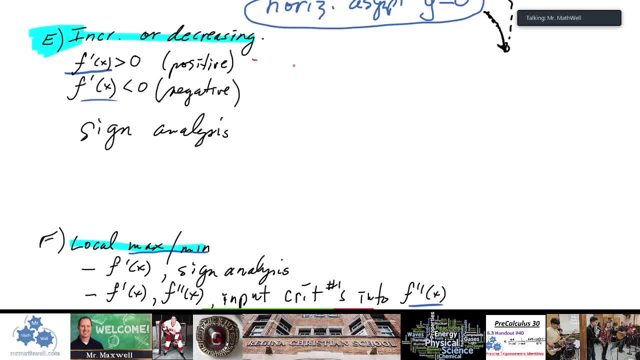 So let's take the first derivative and find out where that's positive or negative. So y equals 1 over x plus 1.. The derivative of y- So let's do quotient rule- Derivative of 1 is 0 times the bottom. 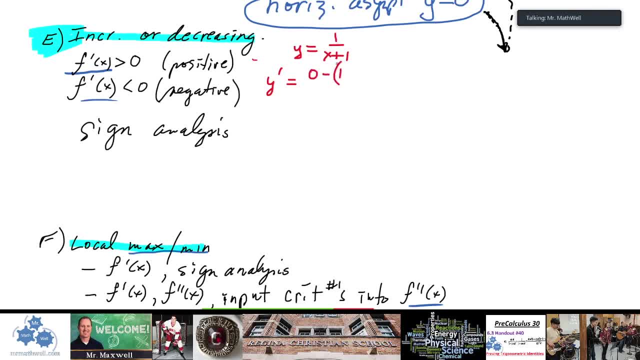 It's going to be 0.. Minus the top Times the derivative of the bottom, Which of course is just 1. Over the bottom squared. Okay, So the derivative is actually negative: 1 over x plus 1 squared. 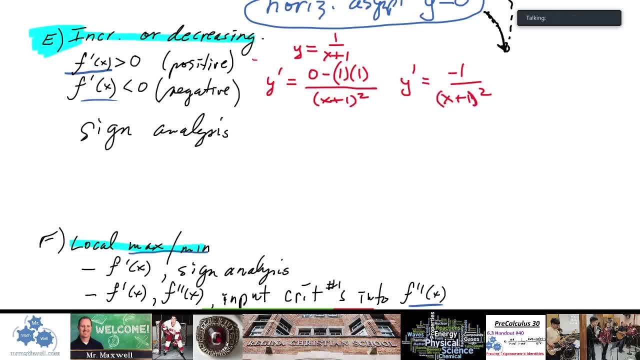 Do you guys agree with that? Does that look okay? Negative 1 over x plus 1. squared Chain rule was just a 1, so we're good with all that stuff, All right, And we need to do sine analysis. Now I've got a negative 1 up top. 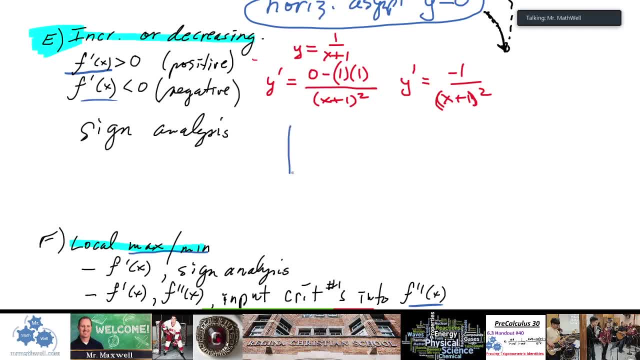 So remember, sine analysis is this elongated L, with all of the factors in the numerator and denominator, And I'm going to put x plus 1 here twice. Okay, Just in case you don't want to write x plus 1 all squared. 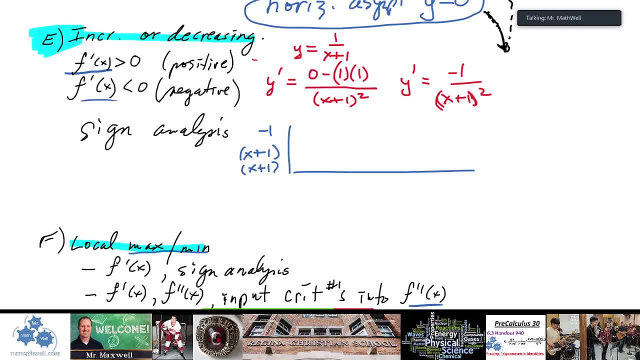 Let's do x plus 1 twice just to make sure, Okay? Sine analysis says that negative 1 is negative all the time. There's no x, so it doesn't change. It's always negative x plus 1.. Is 0 at negative 1.? 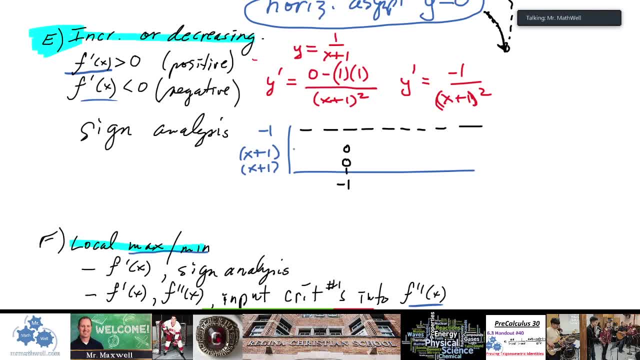 And x plus 1, again the second one also is: It's negative before that for both of these And it's positive after. Whoa, Okay, So y prime then is negative here, Undefined here, because we're dividing by 0 at negative 1.. 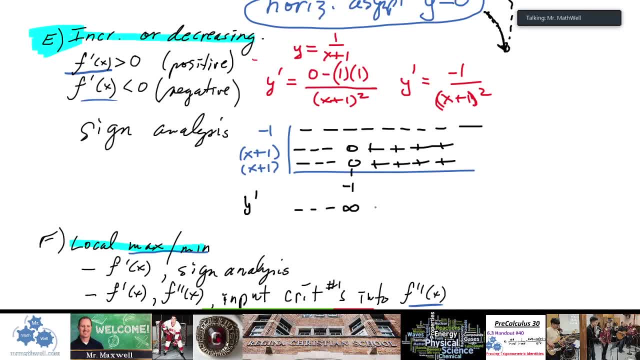 That's bad, And we've got and it's. it looks like it's negative, positive and negative here as well. Okay, So that makes sense, because this is always positive, this squared, and this is always negative, except at negative 1.. 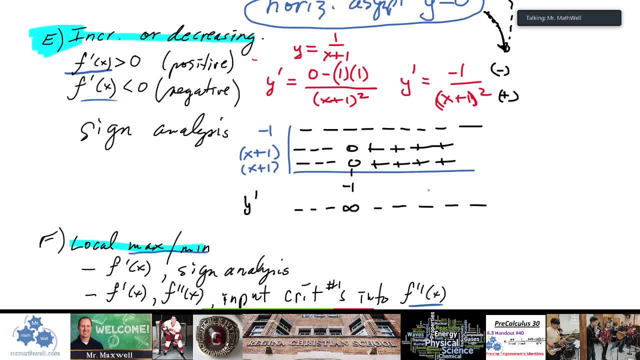 So there we go. That's confirming. So what does that mean? Increasing or decreasing? Well, it looks like the graph is decreasing everywhere, except at negative 1. Which would make sense, because that's our asymptote: Decreasing everywhere. 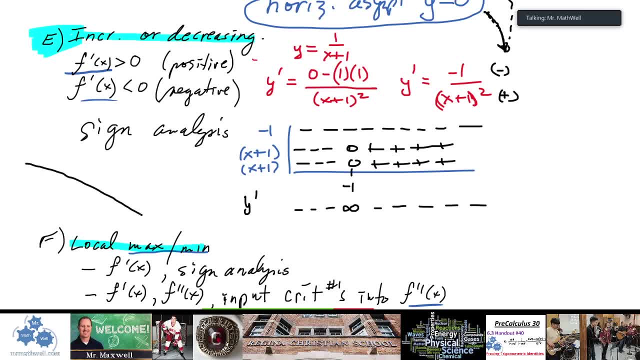 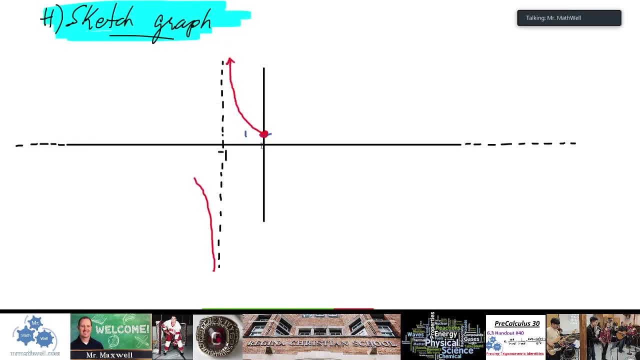 Okay, So that means it's going down always, It's always going down. It never turns around and goes up. So that's going to give us a little bit of a clue here too. Remember what I said before: we have to check to see if something crazy happens here. 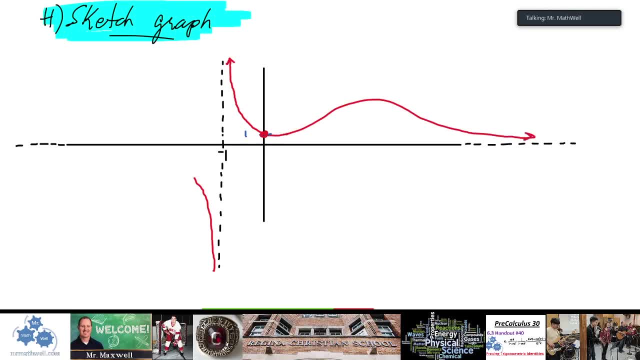 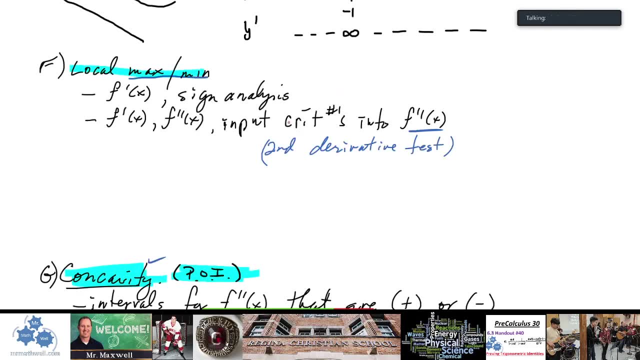 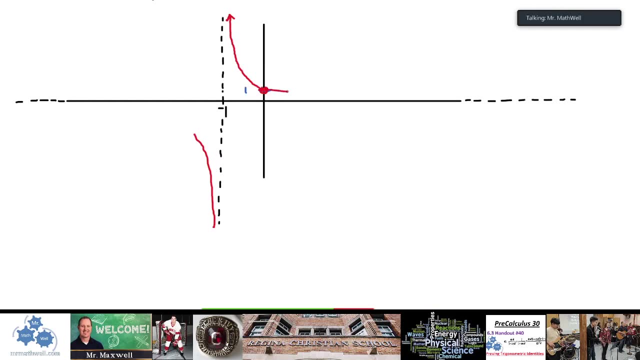 Well, we know this is not the case, because it is never increasing, It's always decreasing. So that's good to know. Let's get rid of that. Wow. So that means that I could probably keep going with this, And it does seem reasonable that this is going to approach this axis, right? 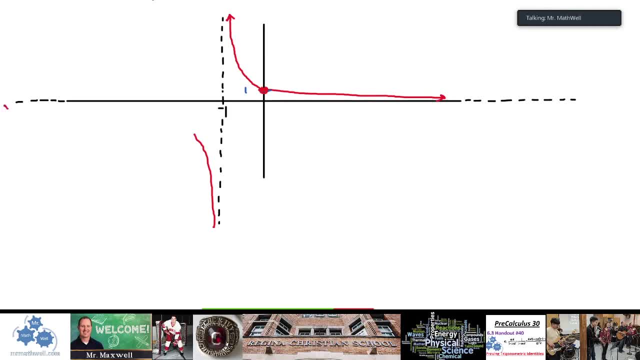 Approach the intercept. And do you know what, If you think about this, if this graph starts up here near this horizontal asymptote and keeps going down, down, down, down, down down. Look at that, It's decreasing everywhere. 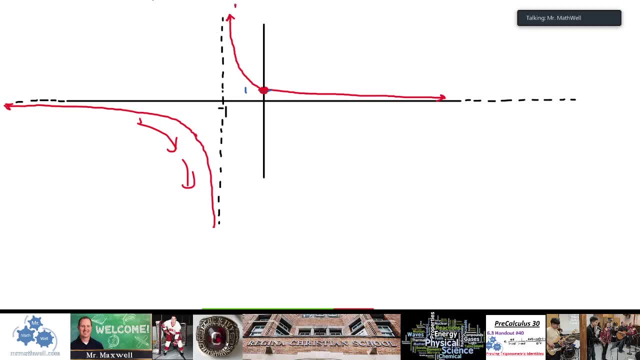 It's going down down, And here it pops up over here It goes down down. See, It's everywhere. So this all should start to be making sense here now, hopefully. Anybody have any questions? All right. 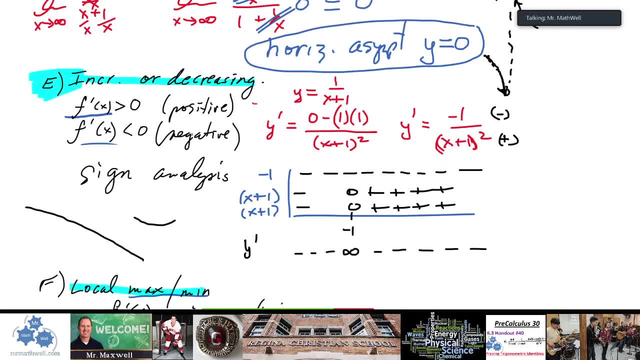 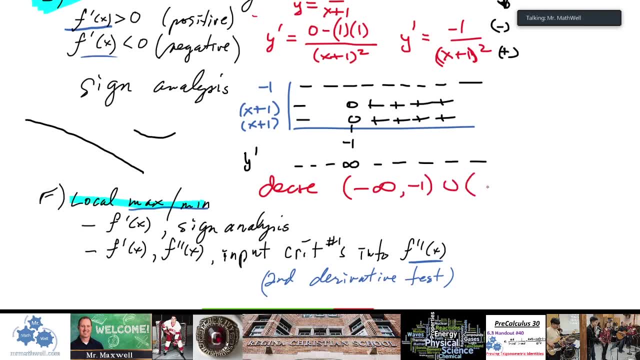 Go ahead and ask out if you need to. So increasing decreasing: We're OK with that. So it's decreasing on negative infinity to negative 1, as well as negative 1 to positive infinity. That's what you would write. So let's say negative infinity to positive infinity. 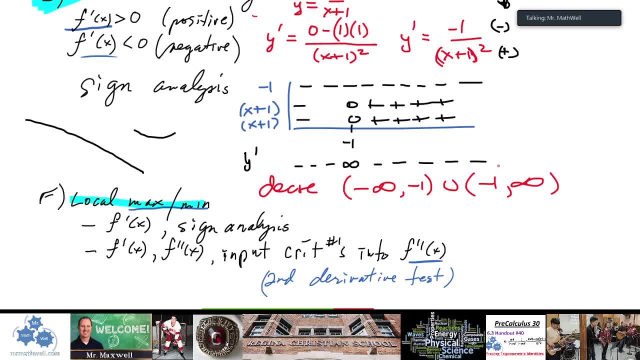 You may see some profs or textbooks say that that's OK, But generally we will not include negative 1 as a point on the interval where this is decreasing because it's not defined. So we will separate that. OK, Got that. 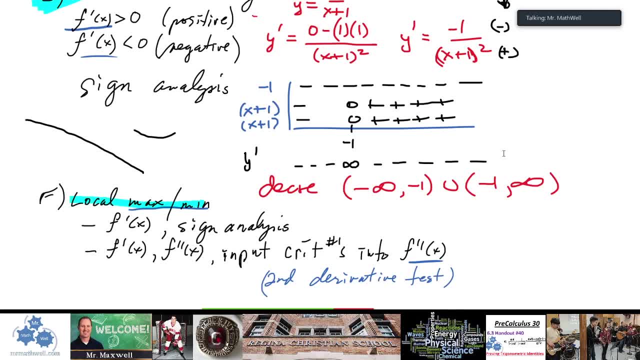 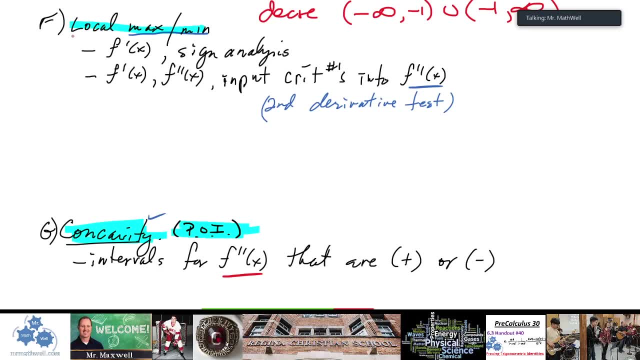 All right, OK, So we're E, We're getting there. F and G: OK, could take a little while, Because now we're talking about local max and mins. So now we have to do some work on the first derivative right. 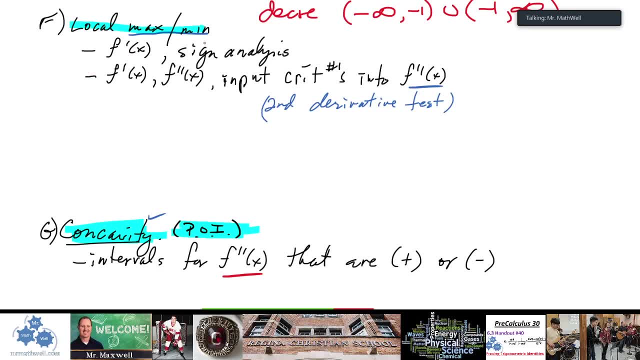 This is what we've learned: First derivative. Now we could take the first derivative and do sine analysis and find out where our local max and mins are, Or we could use the second derivative test. So this is what we just studied, right? 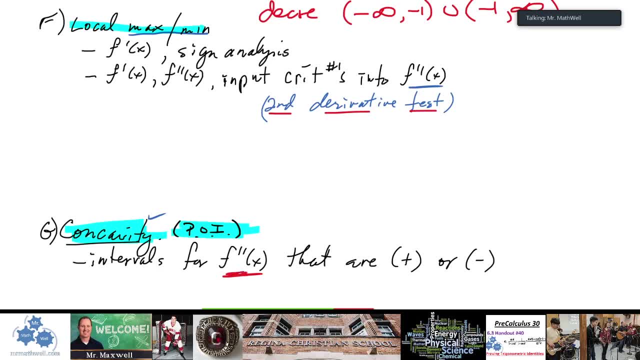 So we're going to have to find the second derivative anyways for G because we need to know about concavity. So I don't know, You can do whatever you want. If you hate sine analysis, then you can just do the second derivative. 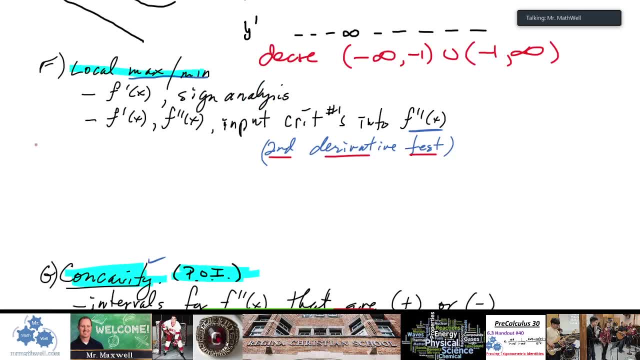 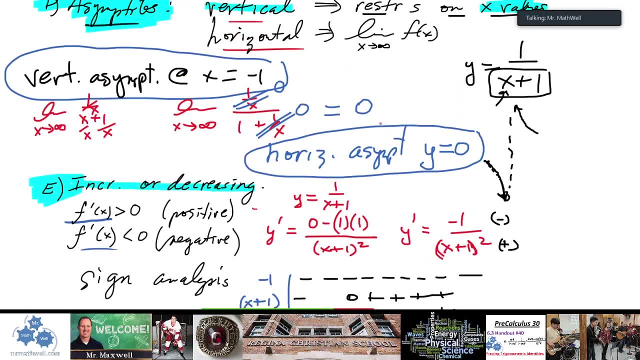 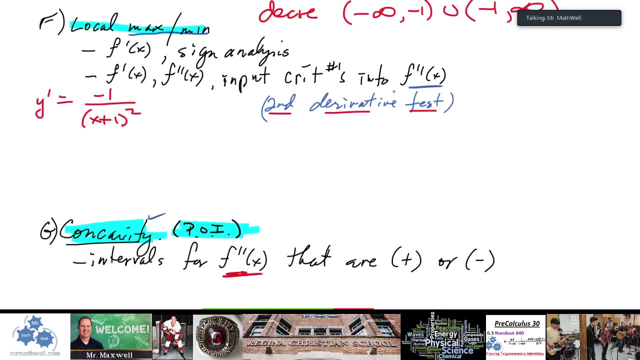 So what's our first derivative? Right Y prime equals negative 1 over x plus 1 squared right. So I'm just going to rewrite that out here. Where did that go? Yeah, OK. Now local max and min. 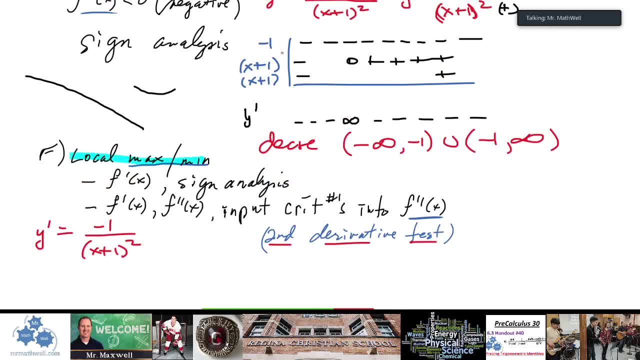 So I kind of did the sine analysis already on the first derivative to find out where the function was increasing or decreasing. So we could actually look back. We could look back here because here's the derivative right. We could look back here and say the slopes are negative here. 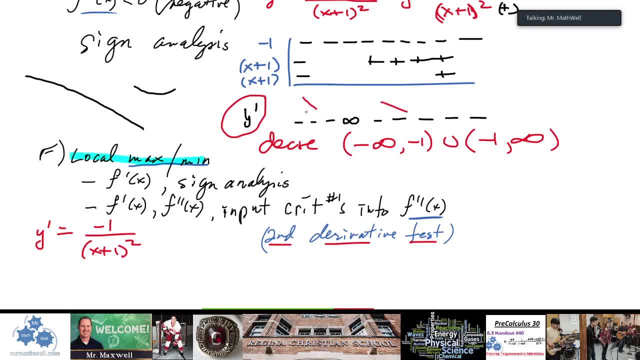 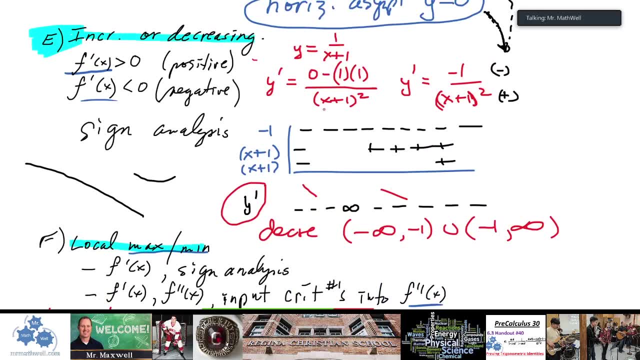 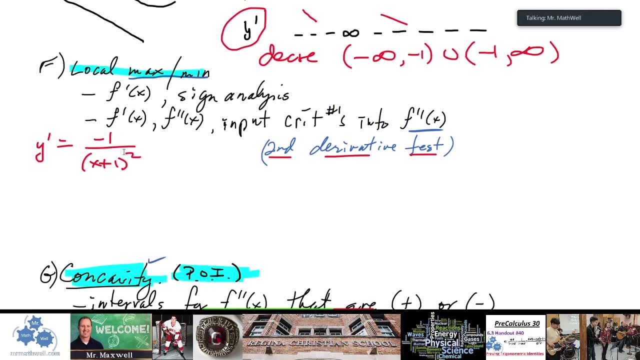 It's nothing there And then it's negative over here, So we don't appear to have a local max or min at all. OK, So if you did sine analysis over here, then you could apply that to the F as well. So let's take this opportunity to do the second derivative test then, because that will also tell us where the local max and min are. 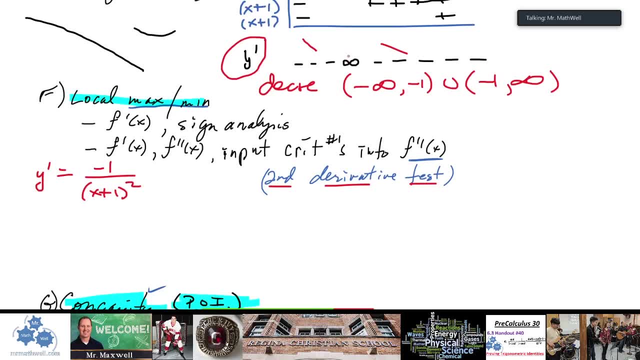 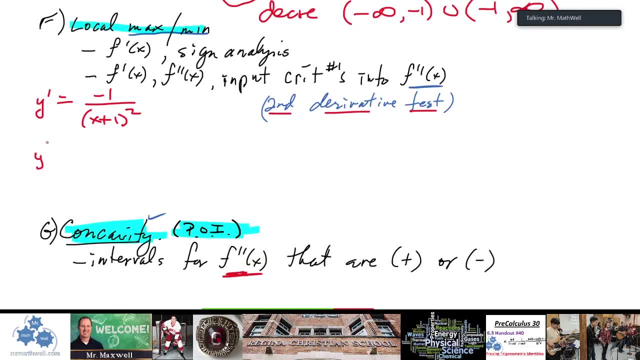 Critical number would be at negative 1.. We kind of already know there's a vertical asymptote, So we aren't going to have any max and mins right. But if we didn't know that we could take the second derivative, And I'll do that, just because we need the practice. 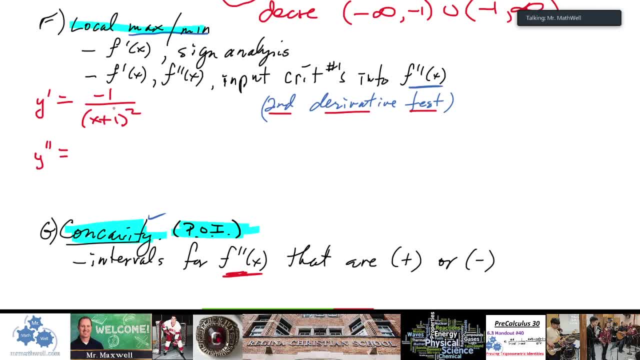 Second, derivative means: we take the derivative of the derivative, So derivative of the top times the bottom is still 0 minus the top times the derivative of the bottom, which is going to be 2 times x plus 1.. So the power of 1, chain rule we're multiplying by the derivative of x plus 1, which is just 1.. 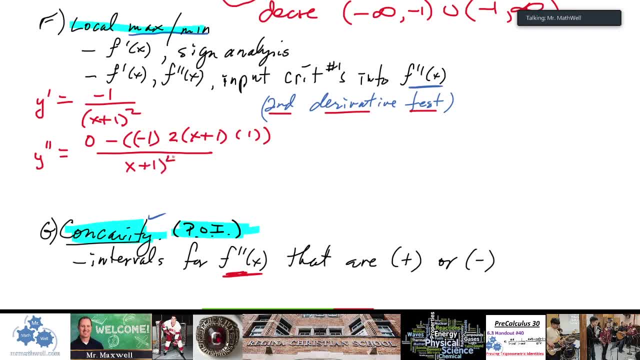 And this over the bottom, now squared. So squared, squared is to the power of 4.. So the second derivative turns out to be: Oh, how do we make sense of all this mess? eh, So we've got 2x plus 2 here, I see. 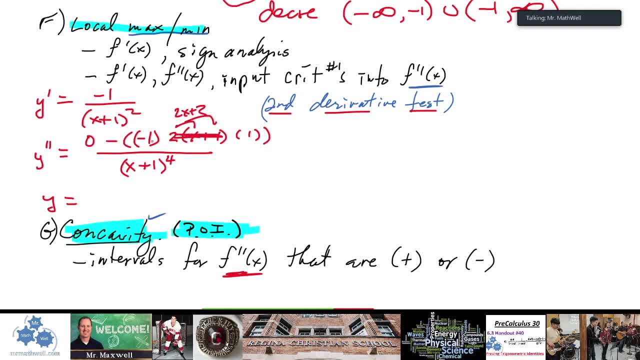 2x plus 2.. And that's multiplied by a negative 1.. So it's negative 2x minus 2.. And we're subtracting that. So we're subtracting a negative 2x, So it's going to be 2x minus a negative 2, which is going to be plus 2.. 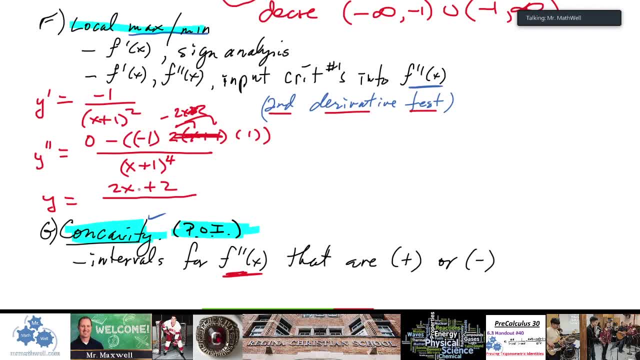 Does that look good? Kind of messy there. Sometimes you can do a couple steps in your head to make things easy, But if you mess up then it sucks. Okay, So is everyone in agreement? this is our second derivative. Are you okay with that? 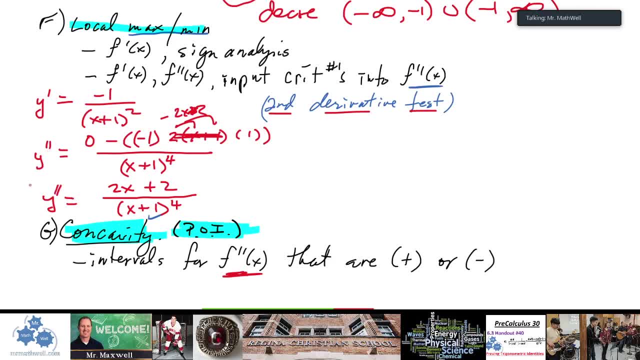 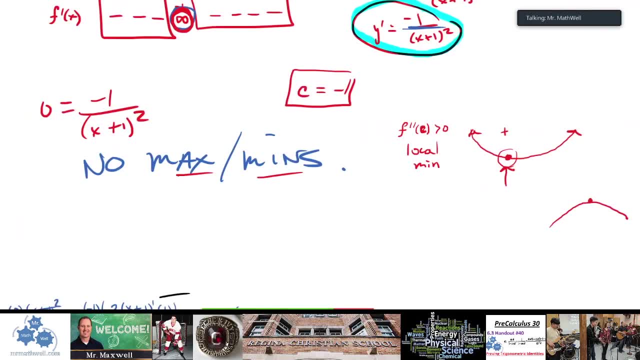 Okay, I really need your help today because I don't have my notes here for this question. I think I have them somewhere else. Let me just check If I was smart. Oh wow, Look at how smart I was, Okay. 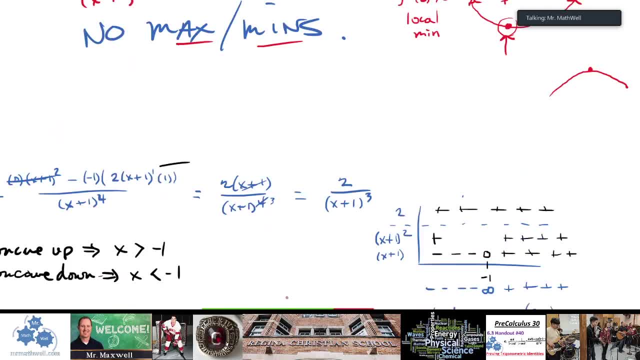 So I do have them over here. I've got them hiding from you. Okay, don't look. Okay, good, I just want to make sure I'm on the right track here. Where's my second derivative? I have no idea. 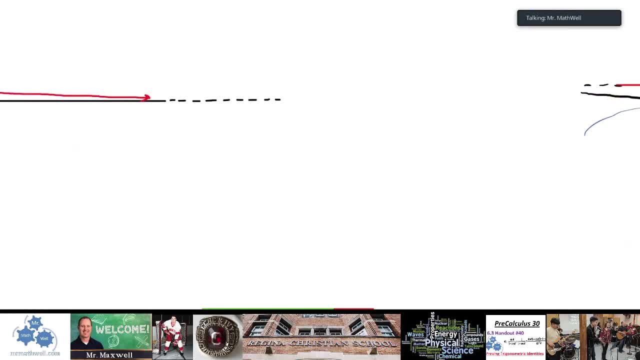 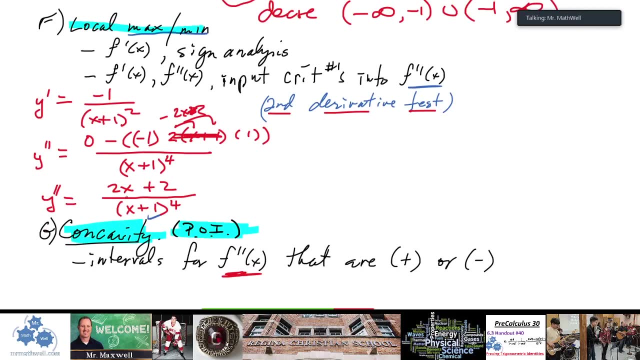 Okay, All right, That didn't help at all. Okay, Let's go back over here. There we go. Resume- Second derivative. So what are we looking for here now? Now we're looking for: We're putting our critical numbers into the second derivative. 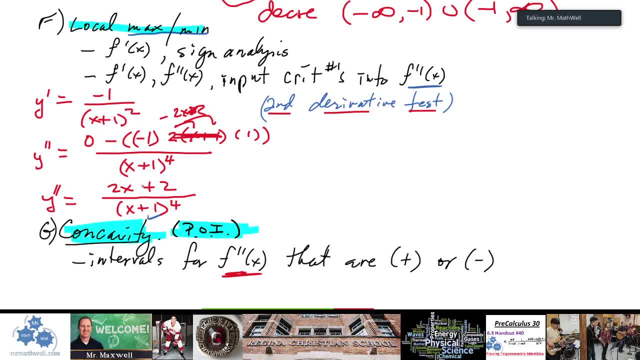 To find out if those critical numbers could be a local max or min. We already know we have no local max or min, because the critical number that we have is undefined. at that point It's not differentiable, It's a vertical asymptote. 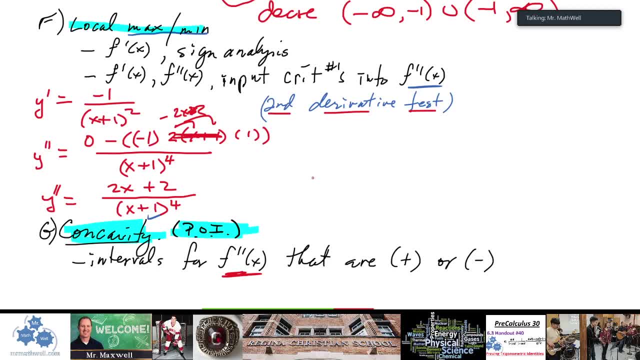 So we don't even have to bother. But if we did, we would put in here negative 1, right, That's what we would do, because that's our critical number. So what happens there? Well, I have 2 times negative 1 plus 2 over negative 1 plus 1 to the power of 4.. 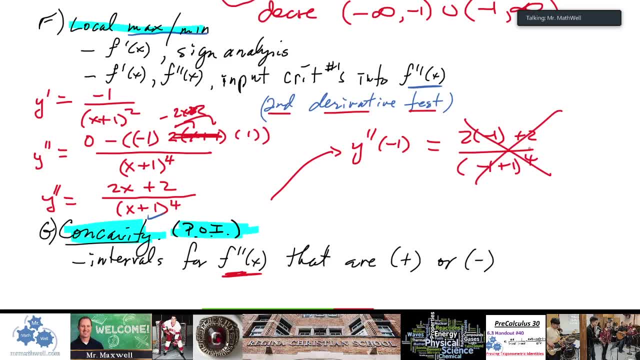 I see that I have zip. I'm dividing by 0.. Boo, Okay, Get no value. So we definitely do not have a local max or min at negative 1.. So you would say no max or mins, No max or mins at all. 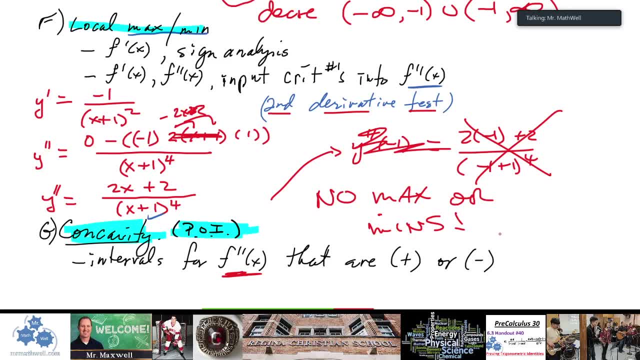 If you did find a maximum or a minimum, you would have to list the point x, y, Okay, So your critical number, This would be your critical number. And then you would say, and you would have to plug this critical number into the original y equation: 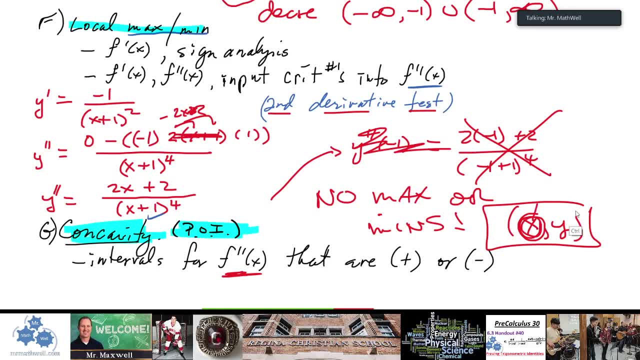 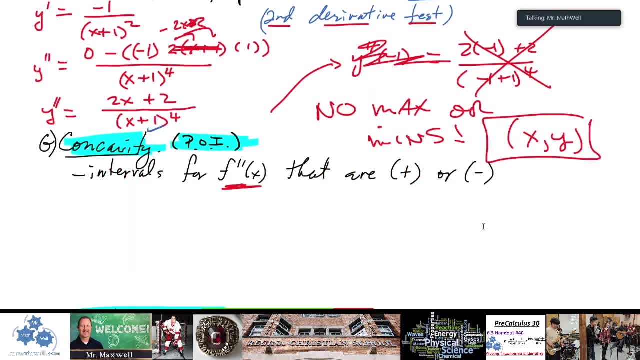 to find your y value. your partner y value Got it. So if there was, you would have to write the point: Okay, Okay, Finally, concavity, All right, Concavity. So now I have my second derivative. I just found my second derivative here. 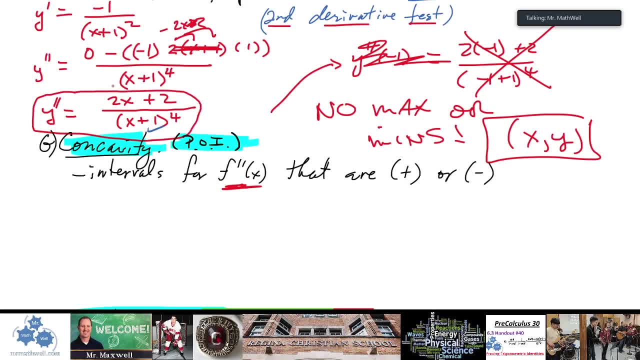 All right, And I need to find out where my second derivative is positive or negative or 0. So let's take a peek At that. So it's 0.. This is 0 when 2x plus 2 is 0.. 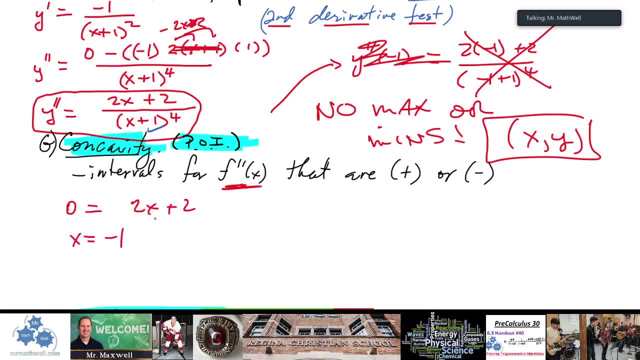 Okay, And that's at. x equals negative 1, isn't it Okay? So x equals negative 1.. We already know a lot about that point. Okay, Does the concavity change there? Well, we should do sign analysis on our second derivative to find out if we have a point of inflection. 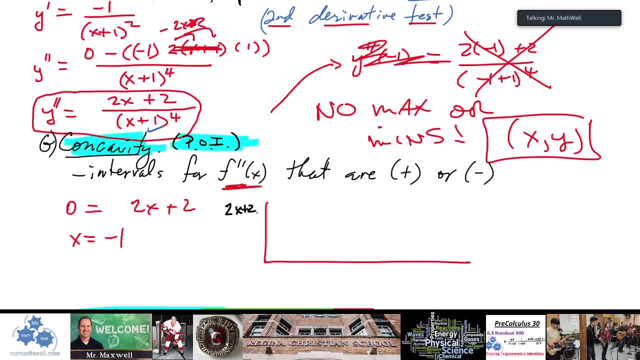 So I'm going to put 2x plus 2.. Or I guess you could factor that and just put x plus 1.. It's going to be the same thing. And then I have my other factors: x plus 1 to the fourth. 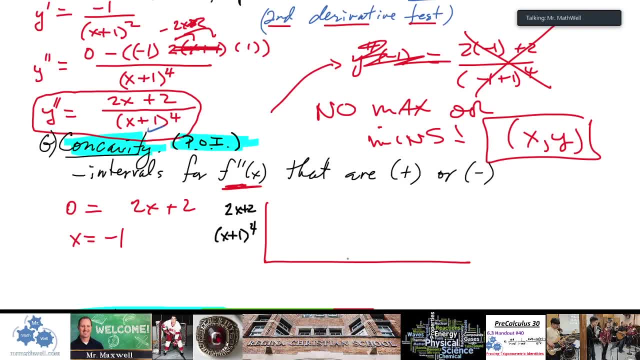 So 2x plus 2 is at negative 1.. We have an issue there. This is 0 here And at negative 1, it's 0 here. But what happens outside of that? Well, this one- because it's to the power of 4, is positive everywhere. 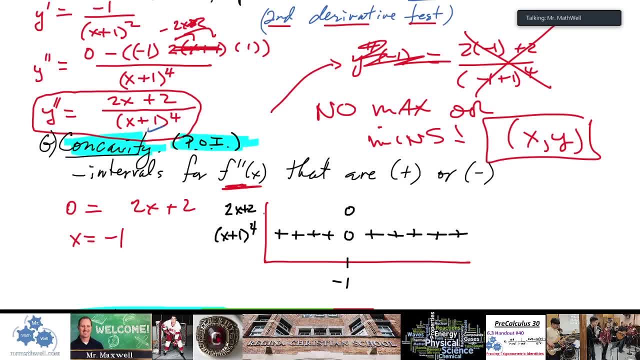 Other than the negative 1, where it's 0. And this now where x is less than negative 1, so like negative 10. That's like negative 20 plus 2, negative 18. So that's going to be negative values there. 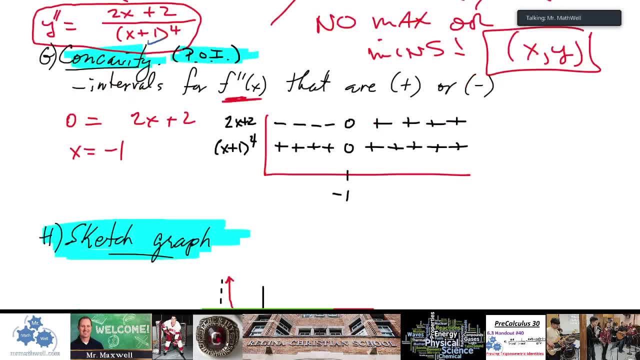 And positive here. Okay, So what does that mean? The second derivative is negative up to negative 1. And it's positive after. So we have the concavity. You would have to state the concavity now, So you would say concave down. 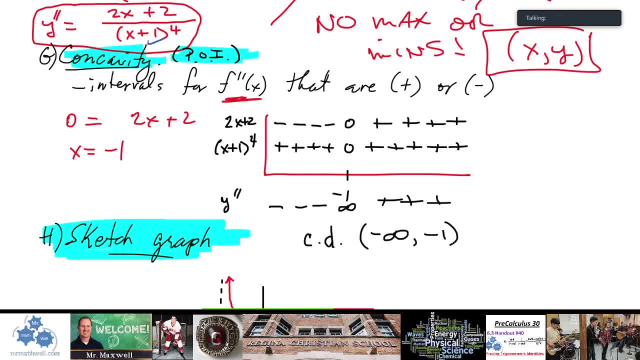 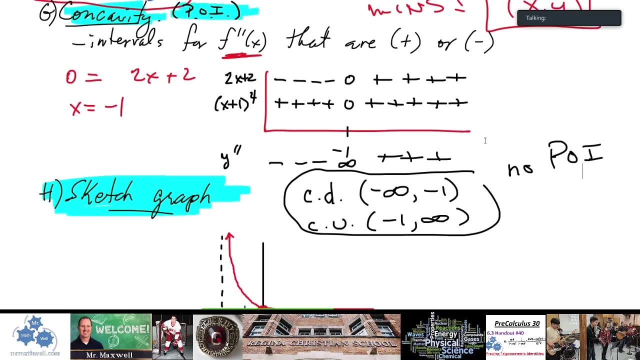 Okay, Negative infinity to negative 1.. And concave up, And I'll let you abbreviate that Cu and Cd from negative 1 to positive infinity. Okay, So that's your concavity, And there's no points of inflection because we are undefined at negative 1.. 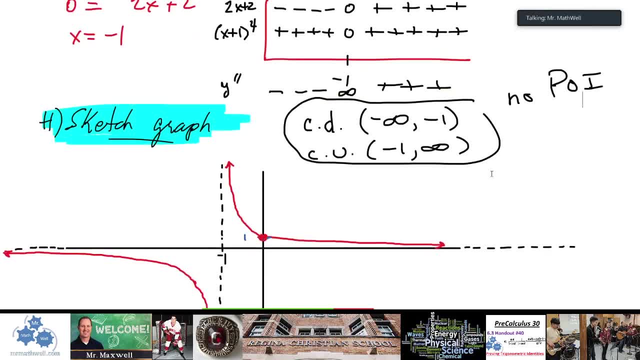 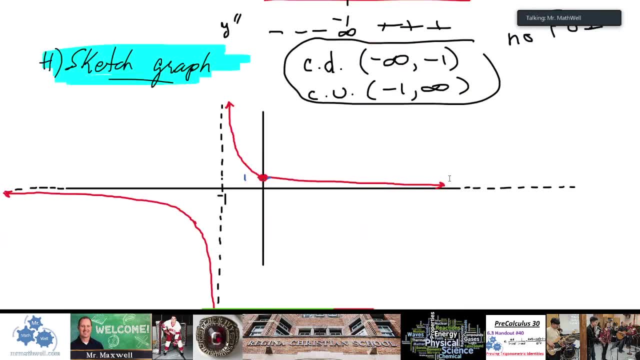 So let's see if that matches up what I've gotten drawn for, Because everything now should line up. That's the last sort of piece. Those are the last pieces of information I need to gather to be able to write my graph here. So concave down to the left of negative 1.. 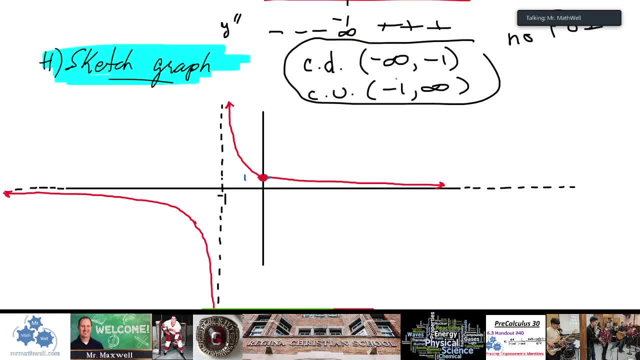 Yep, That checks out, doesn't it Concave up after? Yeah, That does check out, Okay. Even though it seems to flatten out, it doesn't actually flatten out, It's concave up, Okay. So everything checks out. 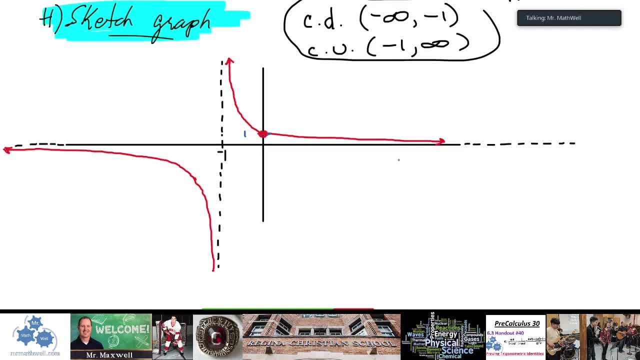 Is there anything else I need to put on this graph? I'm not sure. I think we've done everything along the way, So this is not a difficult graph. Okay, This is our very first example, So I know this is not a difficult graph. 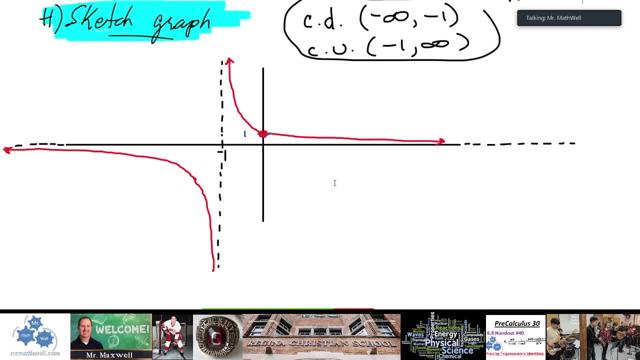 Like I say, we didn't have any max or mins, We didn't have any points of inflection. That's going to take a little bit of work for some other graphs, I will give you that, But for you to understand the process, and this is basically 5.5.. 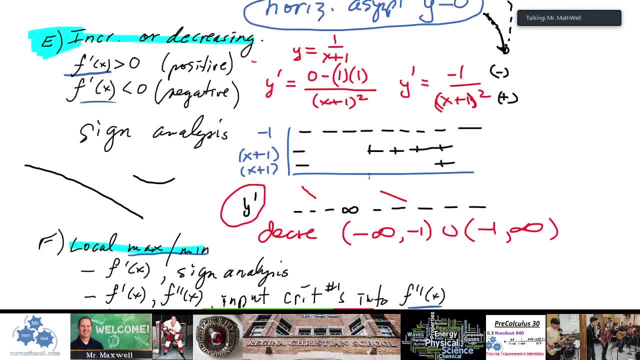 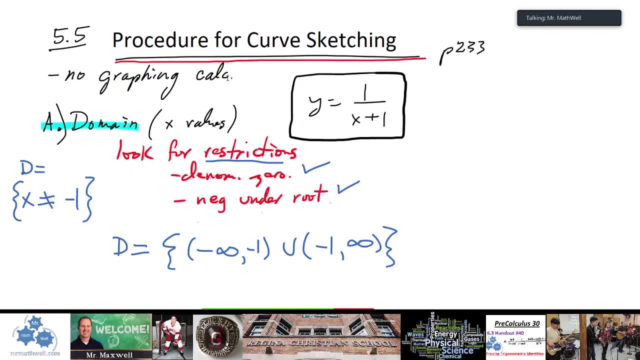 For you to understand this process now. that's everything. Those are the headings A to H, And you'll see in your textbook it'll say: discuss the curve Under the headings from A to H. When you see, discuss the curve, that means do all of this, what we've just done together. now. 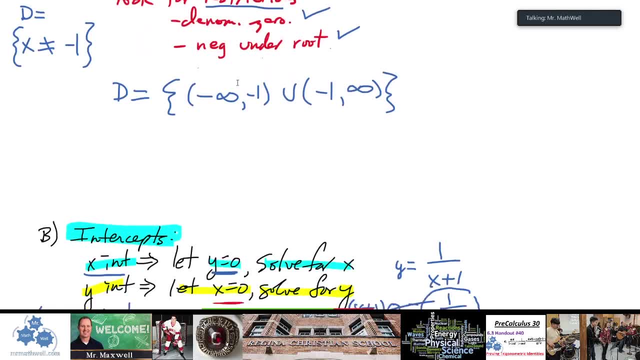 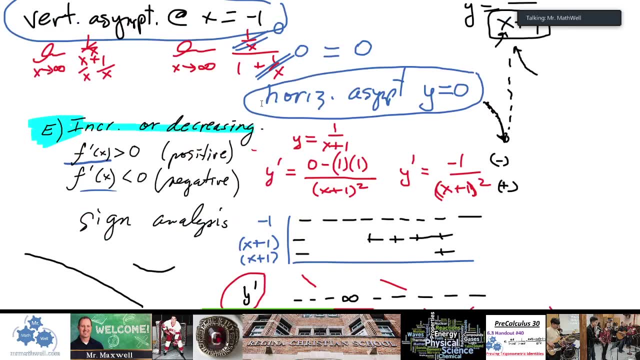 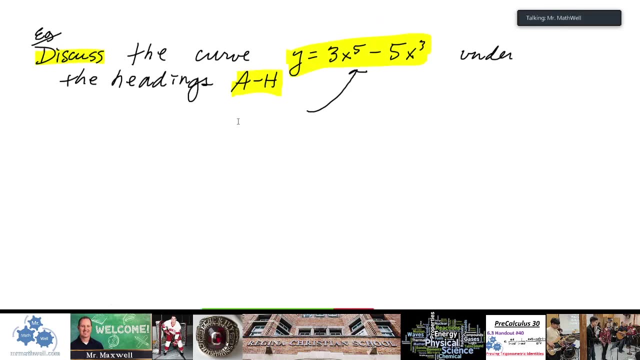 So find out what the domain is, Find out what the intercepts are, So discuss or mathematically identify characteristics for this graph, And then put it all together in a sketch. Okay, Now here's the next part of the lesson. 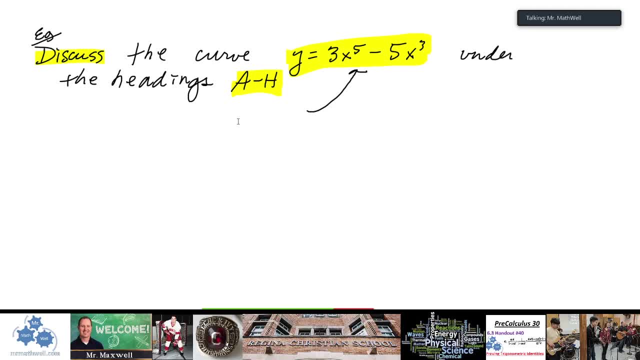 I want you to put this all together for this one And go ahead, and in your textbook you'll see the headings A to H. You also have them in your notes there, But I want you to go ahead and give this a try. 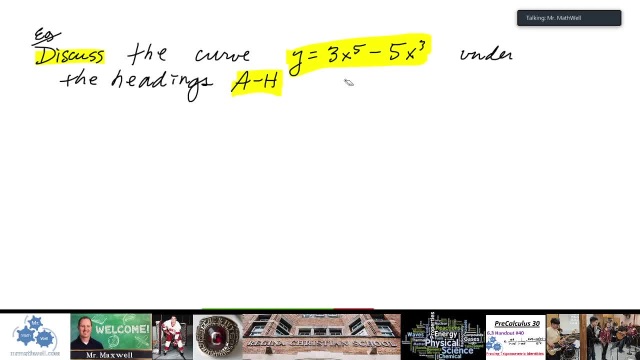 I'm going to give you some time And work through the headings A to H for this one. right here It's a polynomial, So our first and second derivatives are going to be pretty easy. That's nice, But go ahead and work on this for a bit. 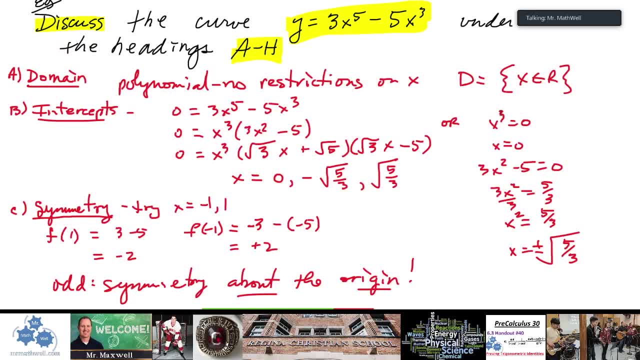 Okay, so just here's A, B and C. If you want to take a look up at the board here, The important things that you should have discovered already is that the domain is XER. It's a polynomial. There's no restrictions on X. 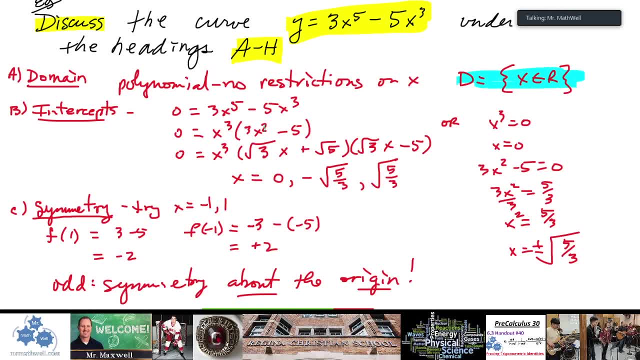 Also the X intercepts. I didn't do the Y intercept, The X intercepts. here are the tricky ones You want to maybe factor- And I factored this as a difference of squares here. You don't have to do it that way if you don't like. 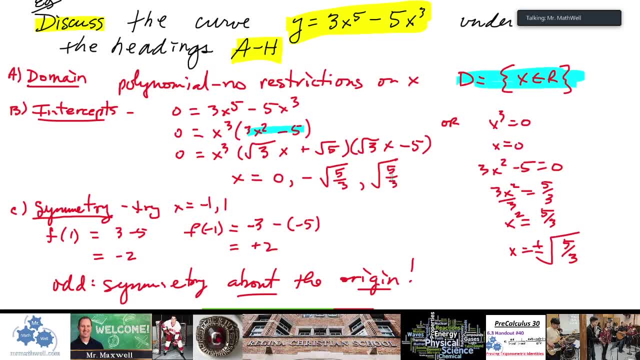 But here's the other way: Just let each factor equal zero and solve. So the X intercept should be: X equals zero, and then positive or negative root five over three, And the Y intercepts, which I neglected to put over here, is simply when X equals zero. 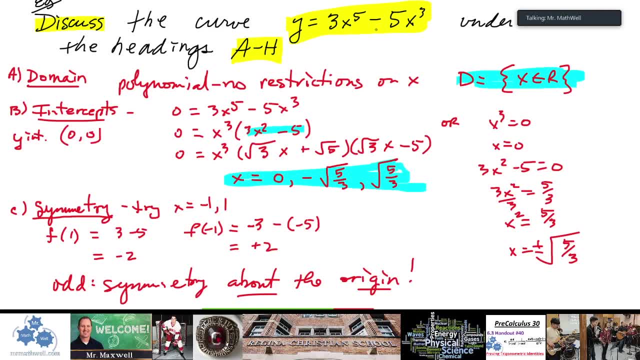 So Y intercept is zero, zero. All right, so just plug zero in there and just get zero, zero. Okay, so those are the intercepts. Now the points. okay, I should write these as points. So obviously that's zero, zero, which is also the Y intercept. 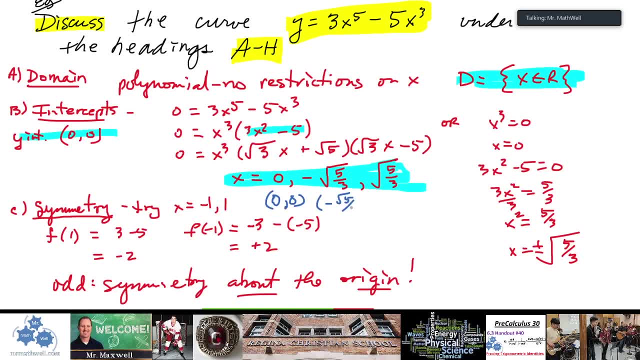 And then it's negative root, five over three comma zero and positive root, five over three comma zero. Make sure you remember we're going to put those points on the X axis. And then the symmetry. I tested the symmetry. Try a positive and negative of the same number and see what you get. 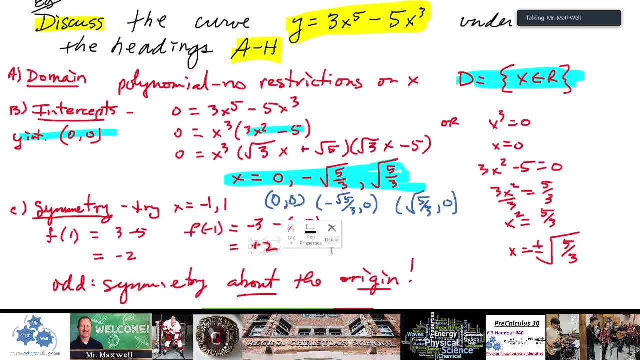 And I ended up getting negative two and positive two. So if they're opposite signs but the same number, then you have odd symmetry about the origin. So these are some things that I know so far for A, B and C. okay, 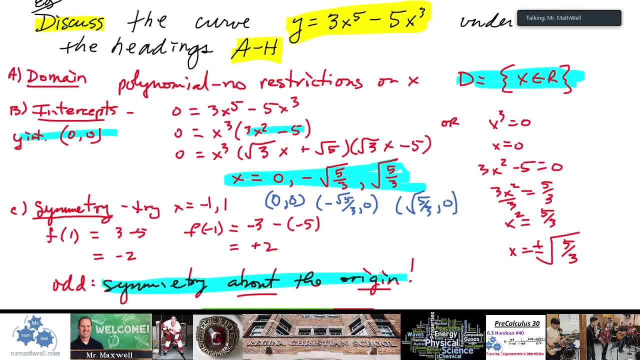 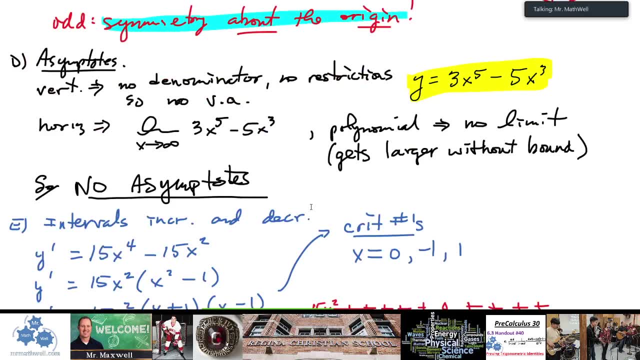 So keep working. Yeah, I'll show you some more in a few minutes. All right, so let's take a look at D and E, then D asymptotes. okay, this is a polynomial, So there's no restrictions on X. 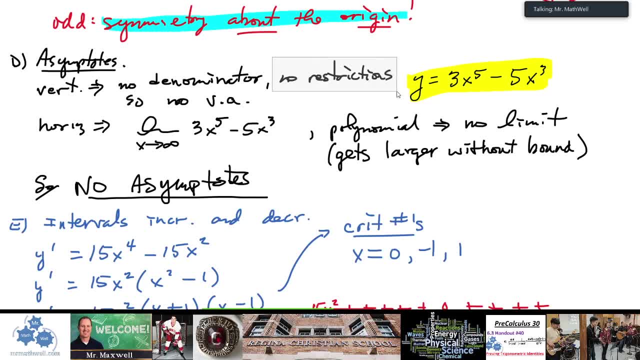 So, if you're looking for X values that make the denominator zero, there's no denominator. So vertical asymptotes: there are none. No vertical asymptotes, no restrictions Horizontal. well, if we take the limit of this function, because it's a polynomial- 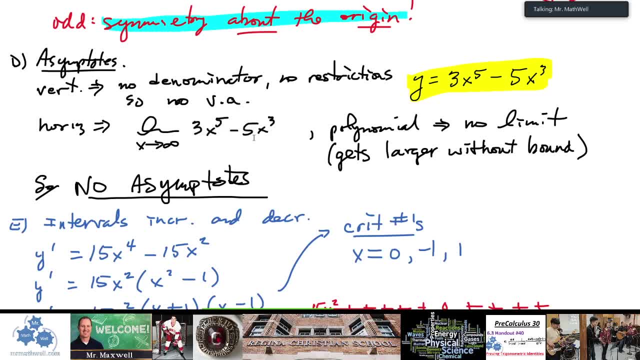 as X approaches infinity, these numbers just keep getting larger and larger and larger. So you have a really large number minus a number that's maybe similar or maybe a little bit different, But that gap is going to grow as the numbers get bigger. So there's no horizontal asymptote. 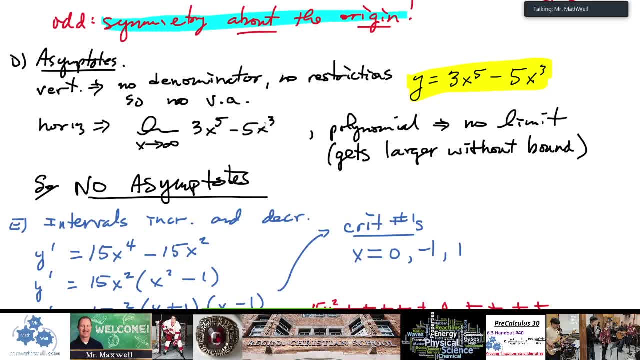 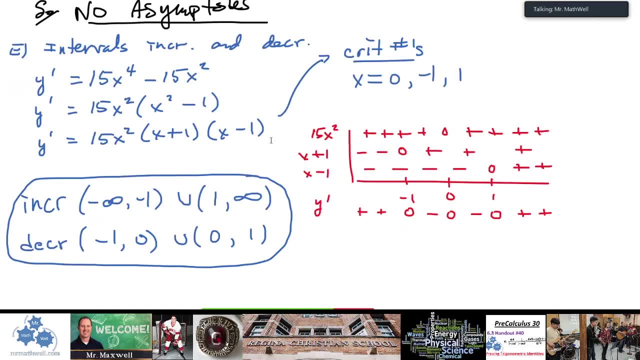 With a polynomial there rarely ever is. It doesn't settle on one number, So there's no asymptotes for D E intervals of increase and decrease. if we take a look at the first derivative right here: and factor that, okay, cancel, factor that, factor that some more. 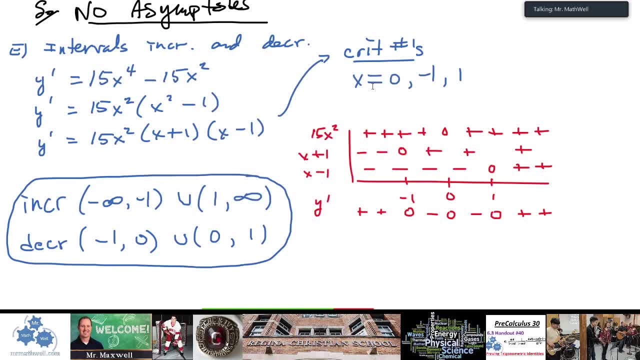 we're going to get three factors And therefore there are three critical numbers that we can identify. if we set this equal to zero over here, right? So the critical numbers would be zero from this factor, negative one from here and positive one from here. 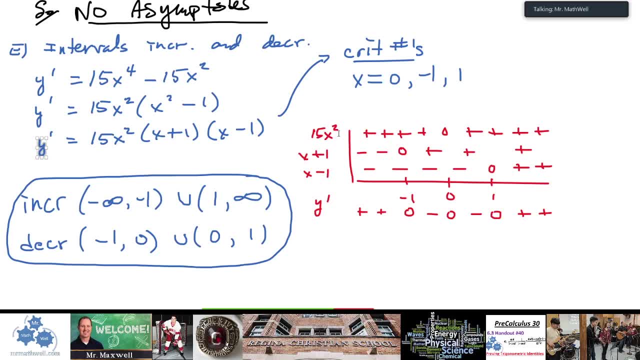 If you set those factors up, do a little sign analysis. the squared term is going to be positive everywhere, except for where it's zero, because it's squared. And then the X plus one and the X minus one will look like this. So our derivative, the sign of the derivative here, will be positive from negative infinity to negative one. 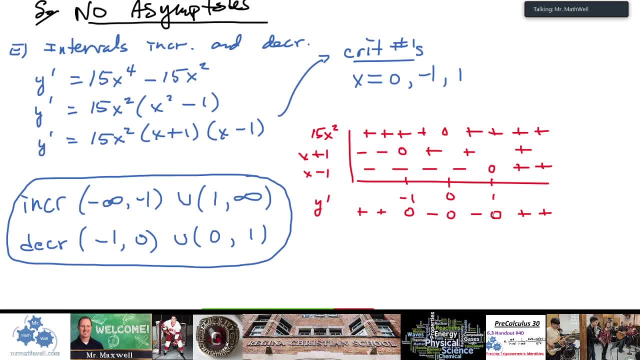 then negative to zero, then negative again to one and then positive. So here's your intervals of increase and decrease for D. So that's what we're looking for in this graph. I haven't been sketching this stuff on the coordinate plane. 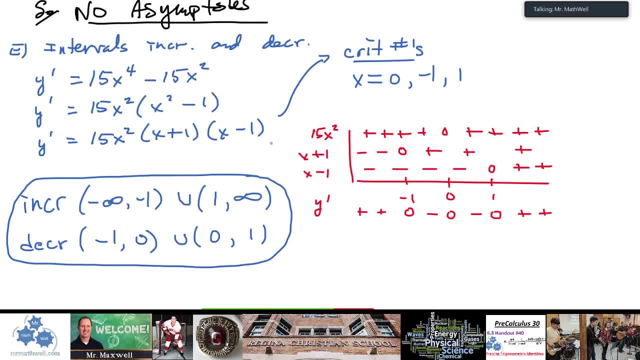 I'm going to leave that to the end, but anyways, maybe you were starting to sketch already and you have a lot of it created, So I'll let you keep working on the rest of it. I'll give you F and G in another few minutes here. 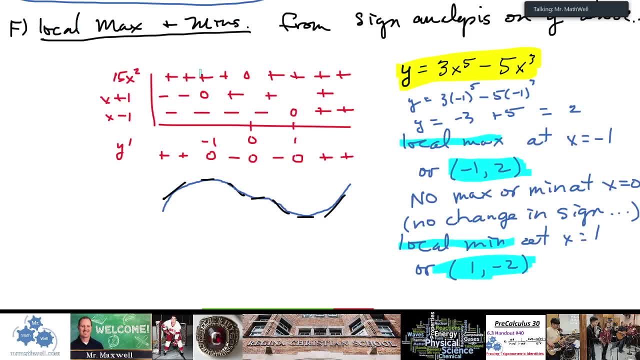 Okay, here's letter F. We already did sign analysis in E, So just borrowing from that we see that we have positive slopes here, up till negative one where there's a zero slope. then we have negative, So that refers to a local maximum right here at X equals negative one. 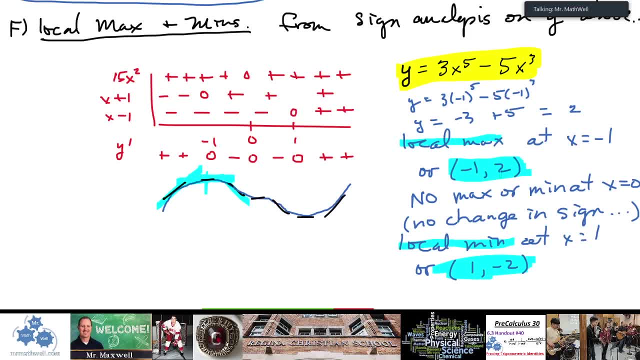 You find the point X equals negative one, so it's negative one. two is a local max. There's no maximum in here. at X equals zero because, remember, the sign needs to change. So we have a negative slope, then we have zero, then we have negative slope. 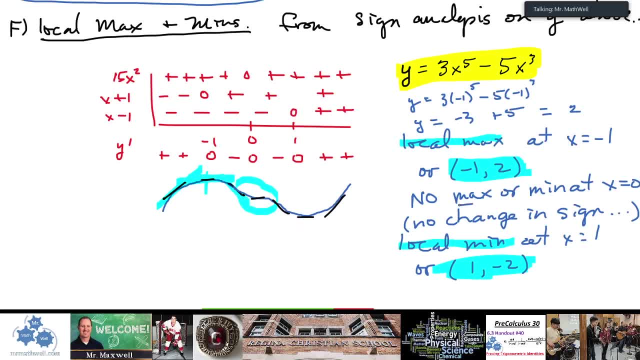 So the sign doesn't change. So we have X or min there and I've identified that here. And then, of course, we have negative slopes, zero slope, positive slopes, so we have a local minimum at X equals positive one. 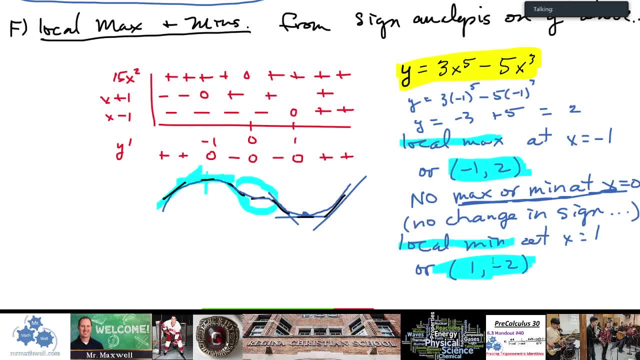 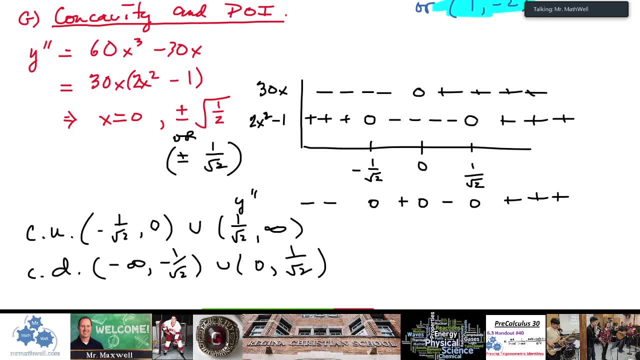 So there's your local max and mins for letter F. So concavity, of course. what we want to do for concavity and points of inflection for point G is to look at the second derivative. Second derivative here is 60X cubed minus 30X. 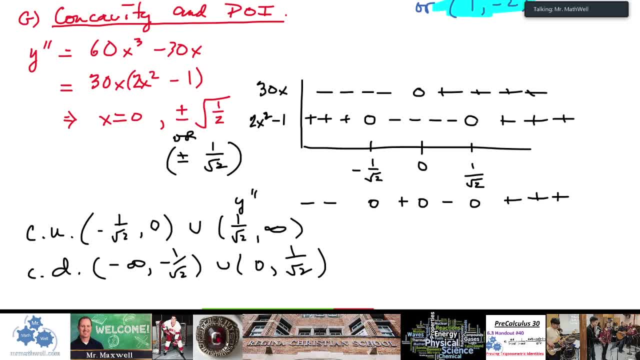 If we factor that, we have zeros. of that, We have zero and plus or minus root, one half or one over root two. Do sign analysis on that to find out exactly where the second derivative is, positive or negative. That's going to give us an indication of what the concavity is and where. 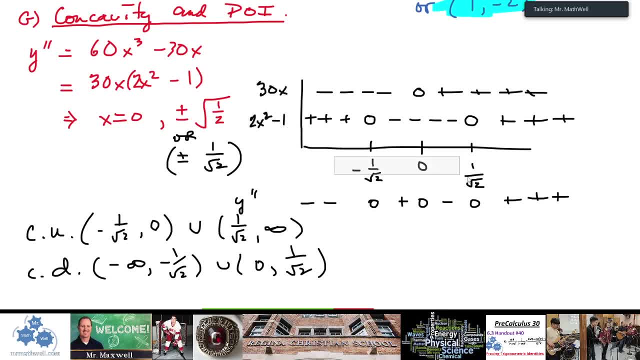 So put the factors here on the left, Do a little sign analysis, Put the zeros down here, And we find out that the second derivative looks like this over the domain. So we are concave up where you see positive there And we are concave down where you see the negatives. 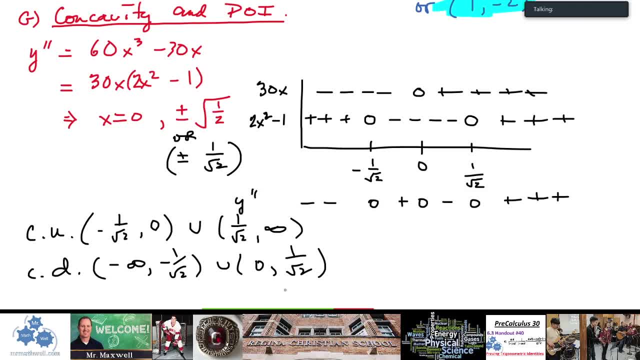 And that's stated right here. And that's the last piece of the puzzle. now for sketching the graph. We're going to be able to do a very accurate job of sketching this graph here. now We have our max mins, We know where our concavity and points of inflection are. 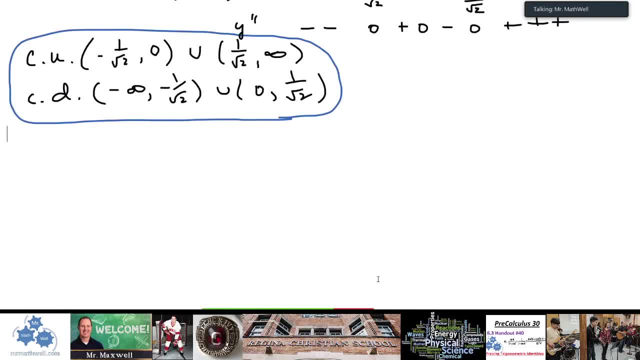 where it's increasing, decreasing intercepts and the like. So for H, we'll sketch here, So we'll put this all together. So the domain is actually R, The Y intercepts. okay, So intercepts, the X intercepts we said were at zero. 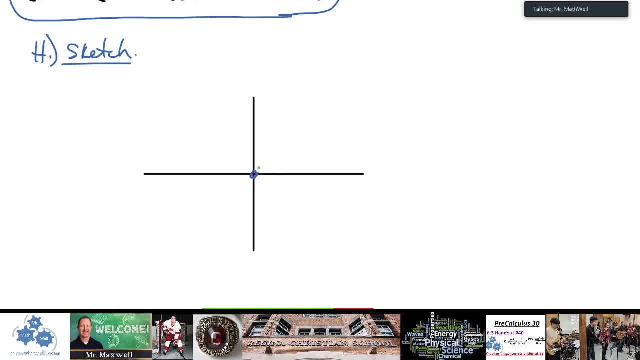 And plus or minus root five over three. So we'll put that on here. So it's negative root five over three And positive root Five over three. So we've got points here and here The symmetry. So we said the symmetry was odd, right. 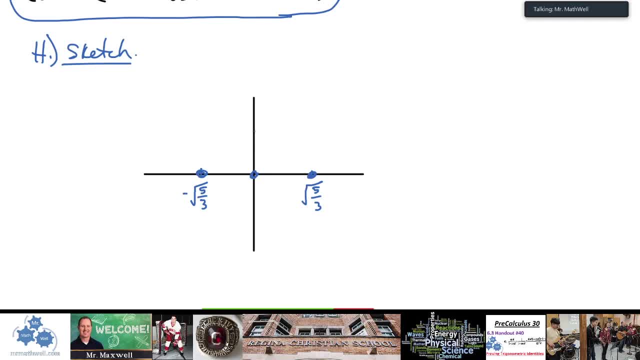 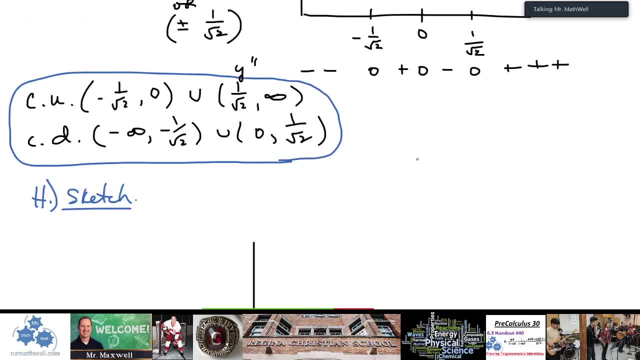 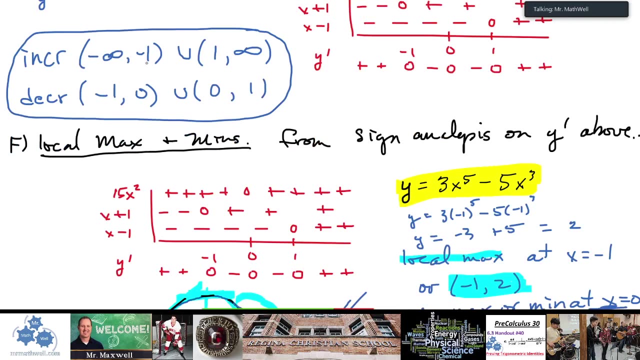 Around the origin. So we'll keep that in mind when we sketch. We can't really do much about that right now. We need some other clues. So intervals of increase and decrease- I'll just go back here. So we are increasing from negative infinity to negative one. 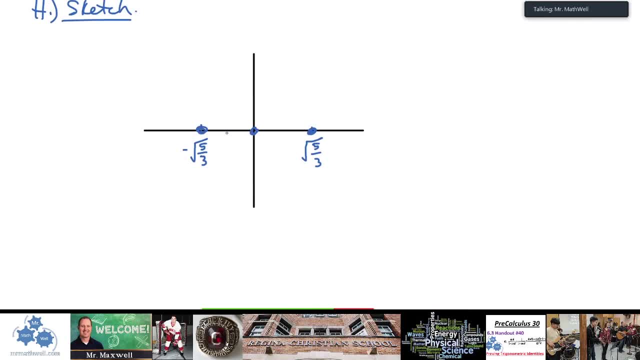 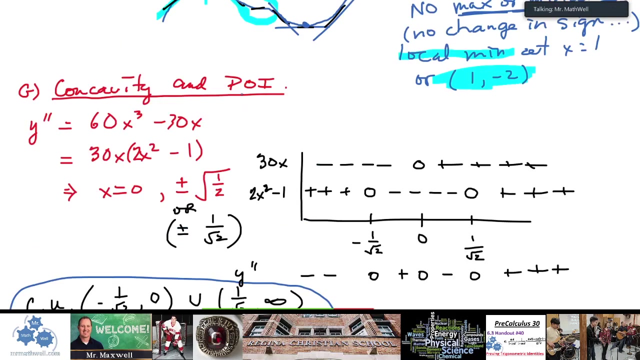 Okay, So we are increasing. We have an X intercept here, So we're increasing all the way to. So negative one would be about right here, I guess, And positive one would be about right here. So we are increasing up to this point where we have local max right. 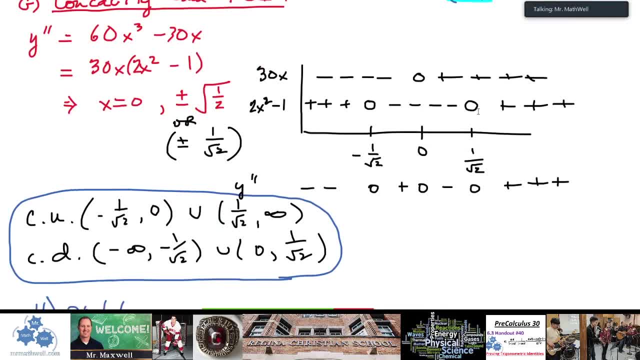 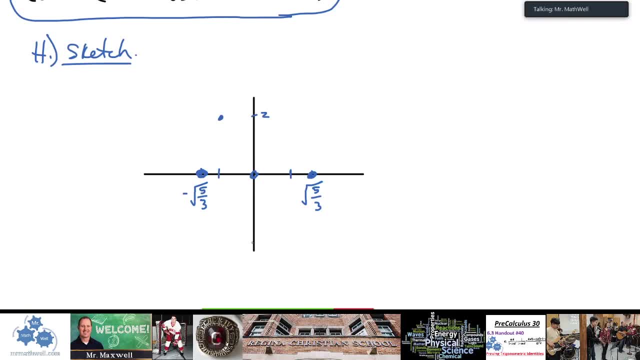 So at negative one two we have a local max. So let's plot that first. So there's two. So negative one, two We have a local max, And at one negative two we have a local min. So we have this kind of thing happening here. 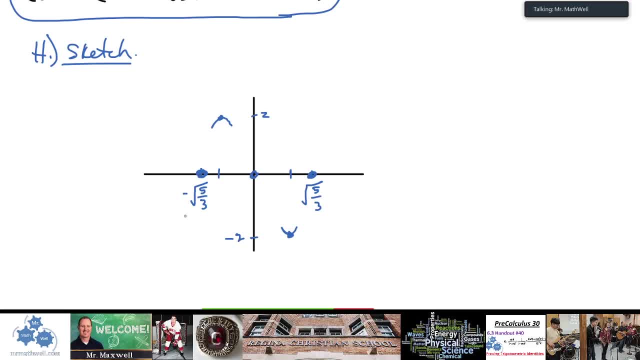 Here and here, Okay, And we're increasing. Now the concavity is the last kind of thing we need to figure out here. So it's concave down from negative infinity to negative, one over three, Negative one over root two, Okay. 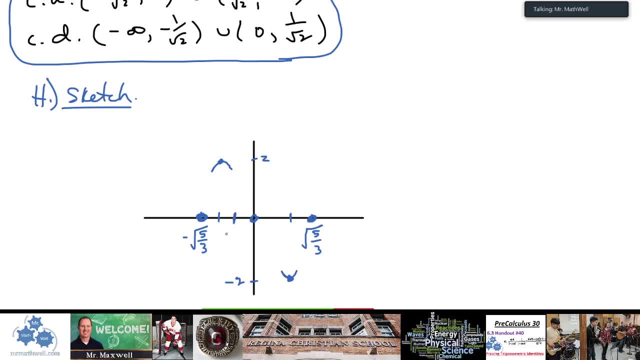 So negative one over root two is going to be right about here. Negative one over root two. And you can figure this out in your calculator too. if you're not sure of where to place these, Just get a decimal form so you know where to place them. 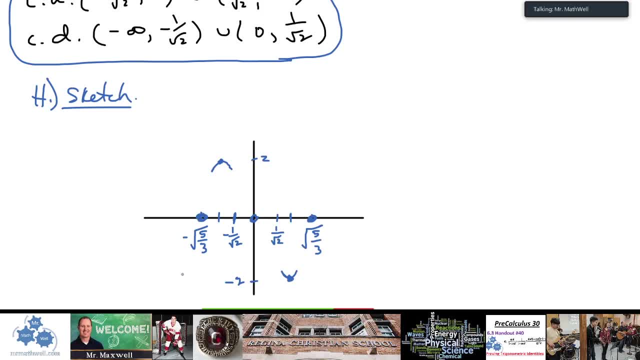 So what that means is you put this all together, Concave down intercepts, Okay, This sort of thing. So it looks like we have something that goes like this, Coming from negative infinity up to here. This is a local max. 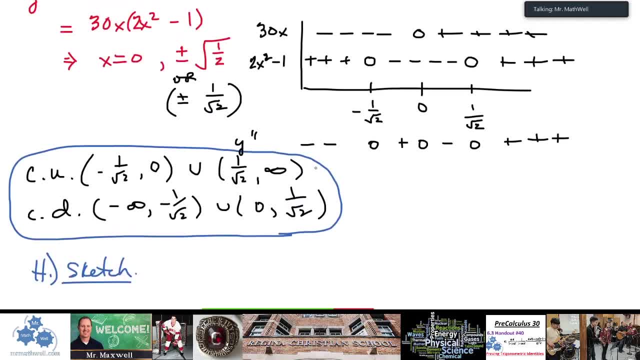 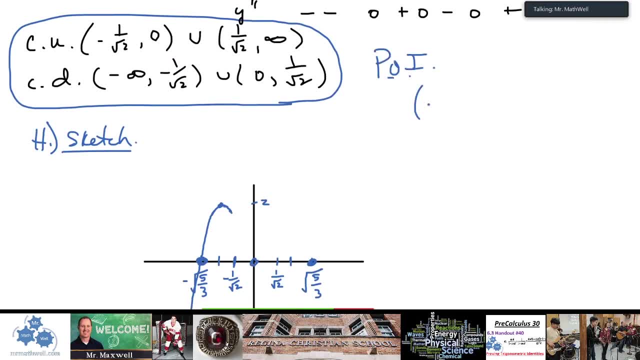 Concave down all the way to. And did I finish my points? Oh, I didn't finish my points of inflection, Sorry. So points of inflection Do need that. So obviously I have negative one over root two When I plug that into my equation. 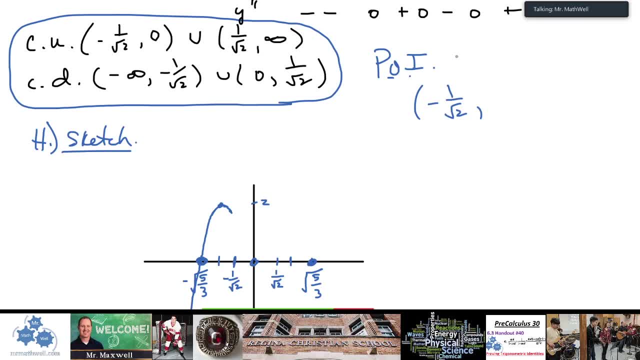 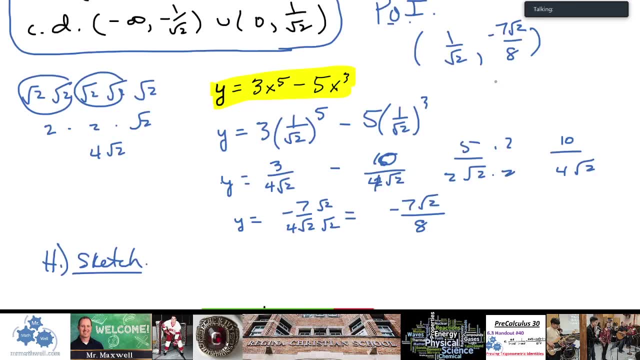 Let's see. Oh, might have to pause and do that. Okay, So here's the work for this. Now, this is exact form. Can you use decimals? Absolutely? Yeah, you probably can To sketch it, But to get points of inflection, though, technically we should. 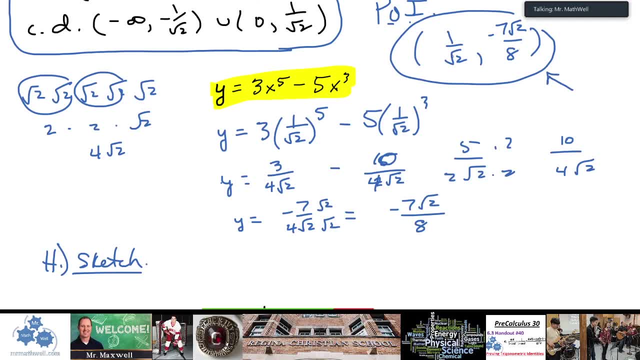 We are looking for absolute or exact values, So you do need to be able to do this. To sketch, decimals are fine, to get a ballpark, But to actually identify the points of inflection you will need to show the exact value. So I'm afraid you will have to do that. 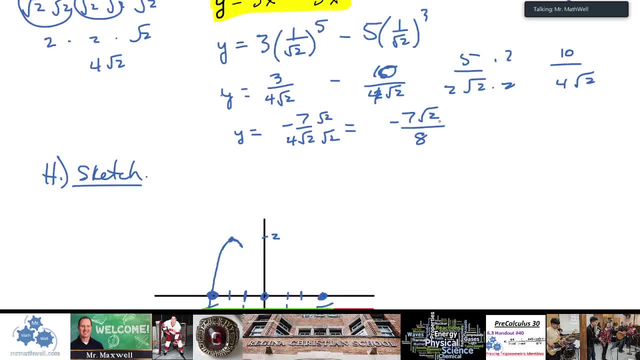 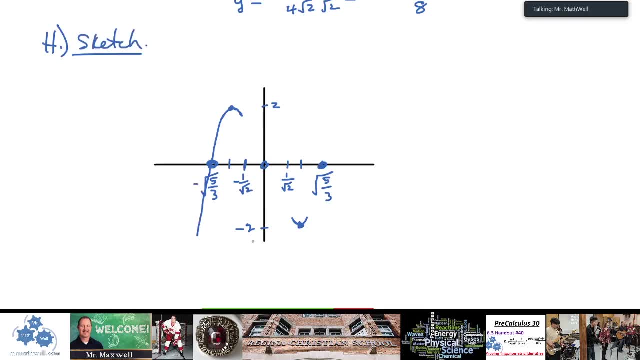 So, at positive one over root two, it's going to be negative. this, Which turns out to be about what did we say as far as the decimal? About 1.2.. So negative 1.2., So it's going to be. this point right around here is a point of inflection. 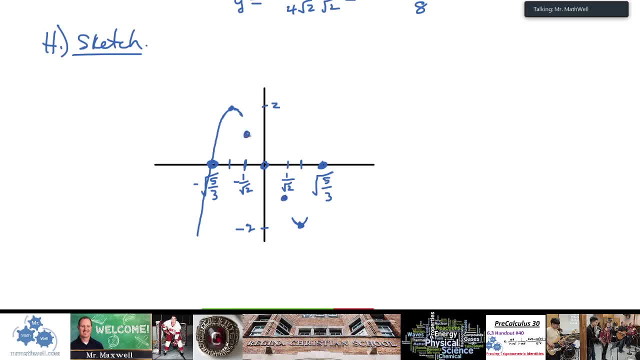 And this is symmetrical, remember. So we're going to have a point of inflection over here. So this is going to be concave down as before, Concave down to here, And then it's going to flip to concave up ever so slightly. 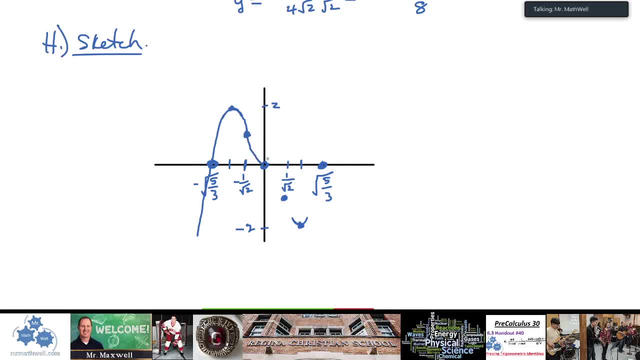 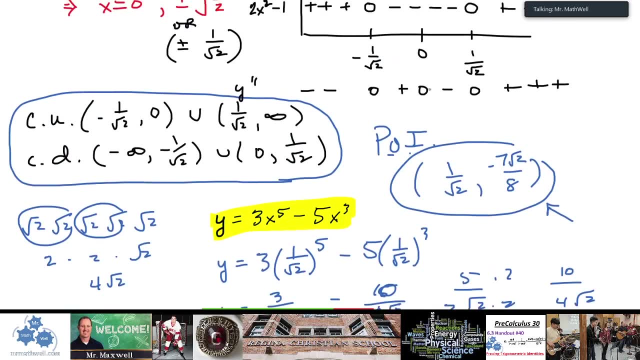 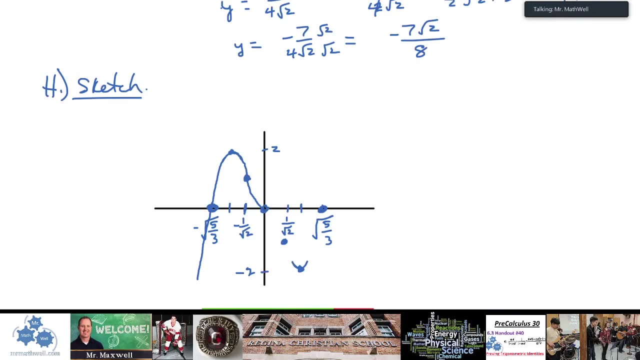 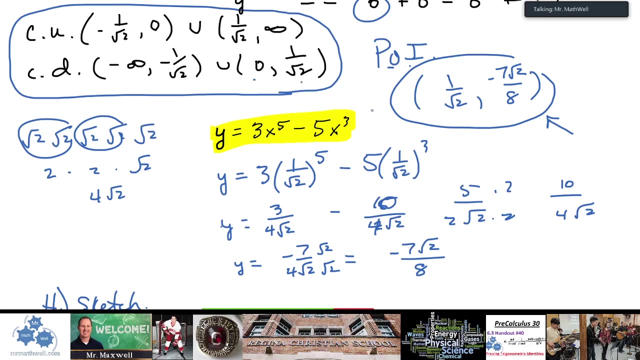 Concave up. Okay, We also have a point of inflection at. x equals zero somewhere, right. So here here and here, So at zero zero. So it's going to go concave down now To match with this here: concave down from zero to there. 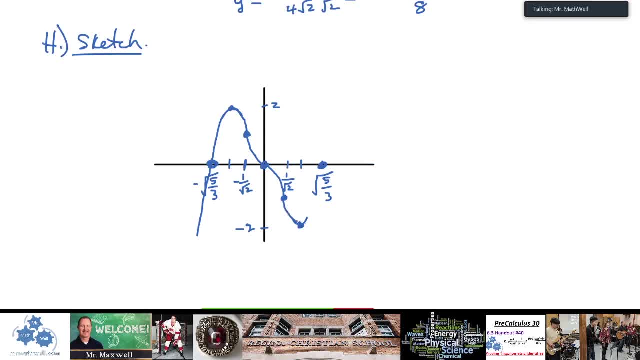 And then concave back up again, Coming to our local min down here, And then concave up all the way through Our x intercept. So it's symmetrical about the origin. It means you could take, literally take that graph. If you could spin it around the origin, it would map exactly onto itself. 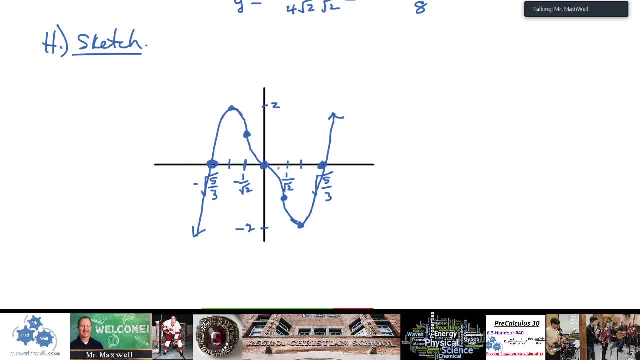 And there you go. That is a very good, accurate graph of this, And we really would have no hope of doing that without the calculus, Unless we just plugged it into our graphing calculator Right. So again in calculus 30 and curve sketching like this: 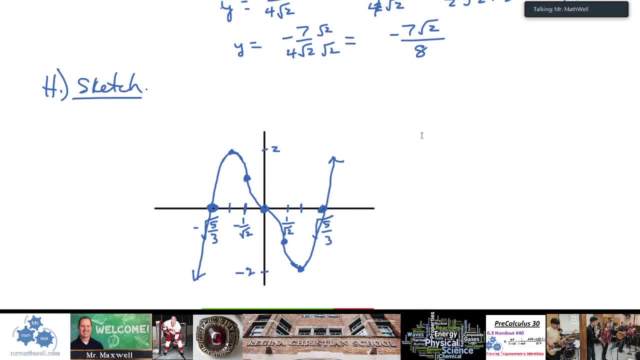 Yes, we have technology to do calculus. That is not, you know, a secret, But when you're learning calculus, when you're studying calculus, you have to work through by hand how this stuff works so that you more fully understand it. 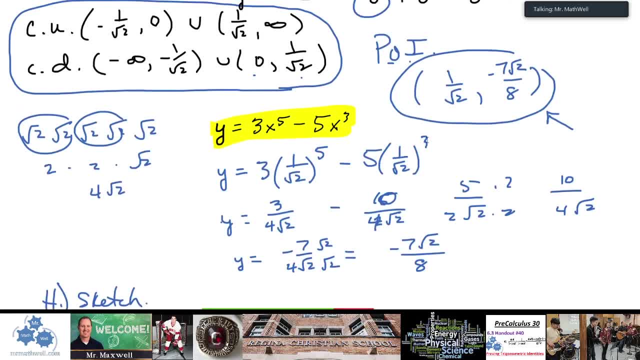 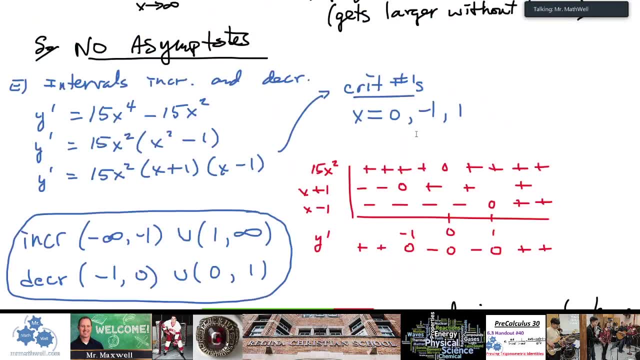 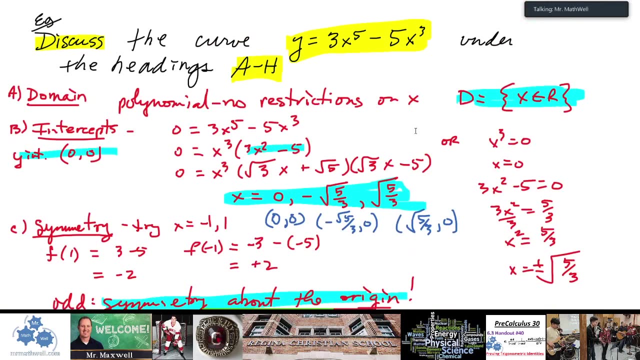 Okay, So the fact that we can use these calculus, use the calculus to determine characteristics of graphs and then go ahead and sketch that very accurately without using technology, is sort of the goal here, Right? It's kind of like the pure math, This is pure math. 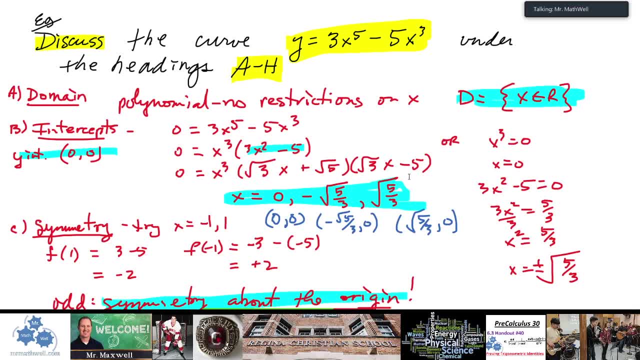 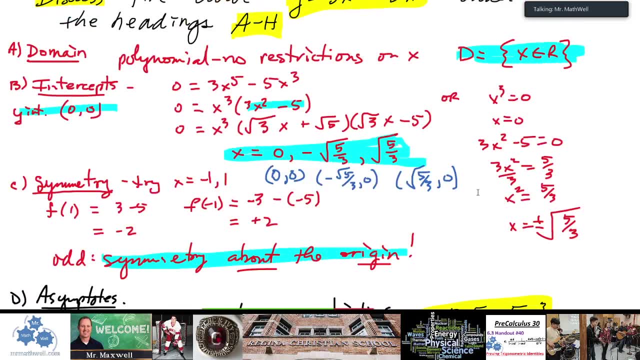 You're investigating this math and you're doing it just for the sake of recognizing and capitalizing on the patterns and the math that is available. So good job if you got through that question without pulling your hair out or gnawing your own arm off. 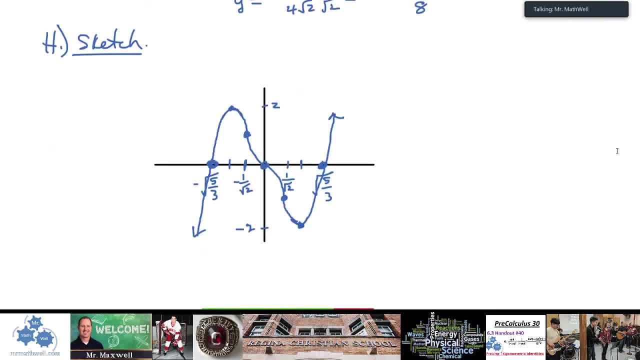 Good for you, And that should be how it looks there. Isn't that beautiful? Now you think about that. What's that? half an hour, 45 minutes of work for that graph- Isn't that beautiful? You should really take pride in that. 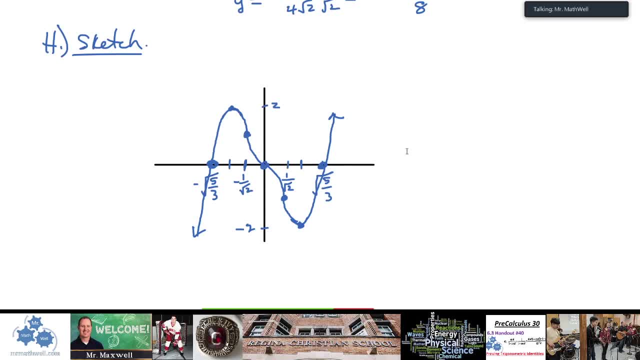 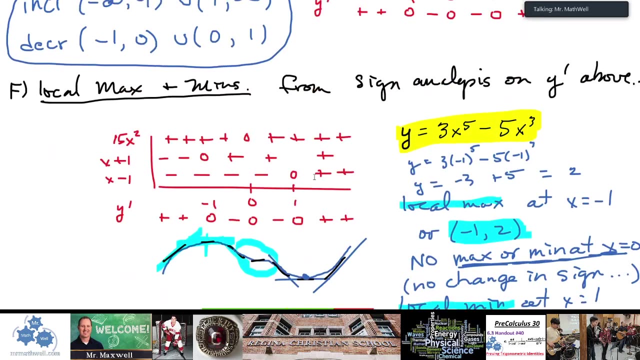 You really should. Yeah, The other thing would be that you should label your max and min points and your inflection points on the graph to make this complete. Okay, So I'll do that, Yeah, Okay, So you want to go back up to F? 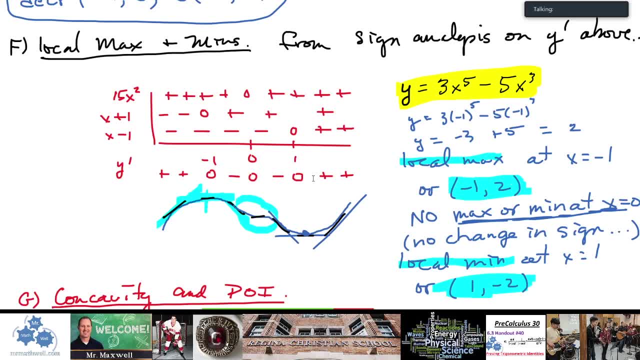 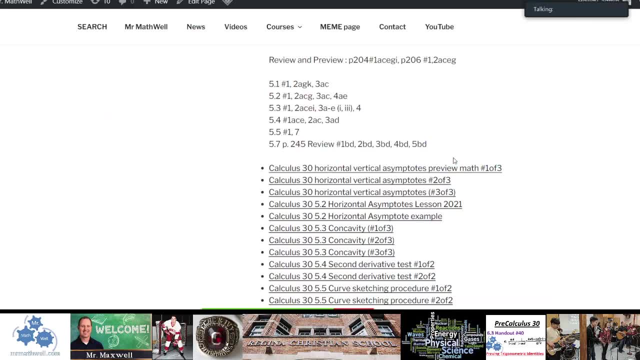 Sure, Okay, While you're looking at that, Your homework for Chapter 5.. I'll show that up on the screen here. All right? MrMathwellcom has all sorts of fun for you here: Videos on all of this stuff, as well as suggested homework assignments. 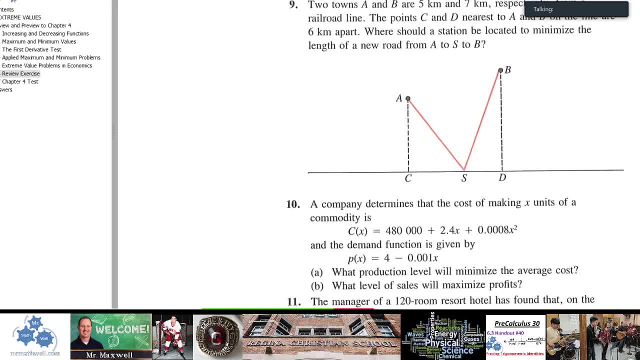 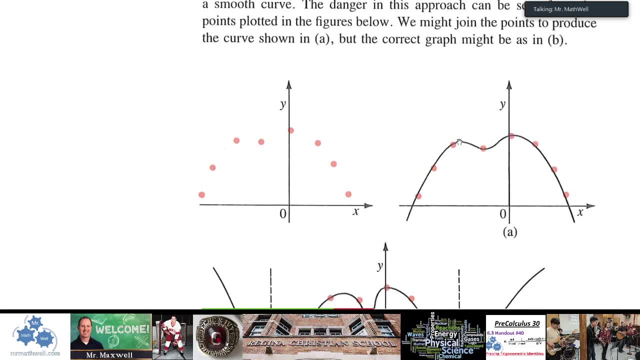 Here's going to be. Oh, wow, Anyways, I was going to show you some textbook here, Hang on. Yeah, So here's 5.5 in your textbook. It's talking about a procedure for curve sketching. There's your.